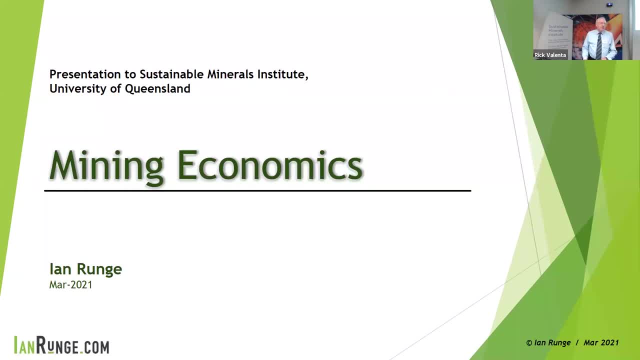 you won't be feeling too dismal at the end of my talk today. Now, I'm assuming my audience are all mining people, if not technical professionals, at least familiar with the industry, and I'm assuming that most attendees are from the mineral processing. 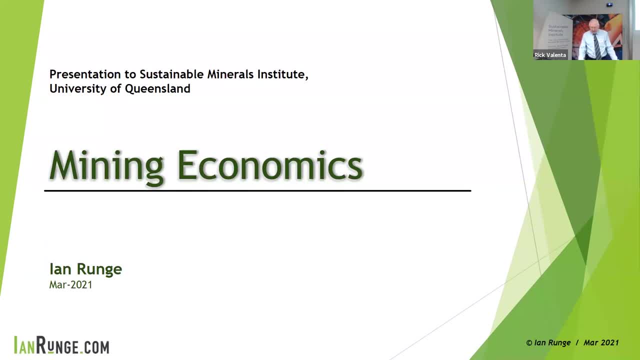 metallurgy end of the technical spectrum- rather than mining engineers or geologists and, I'm assuming, a certain level of familiarity with software and modelling and simulation. The end of my talk today is going to be a little bit more formal, even if it's just on an Excel spreadsheet. 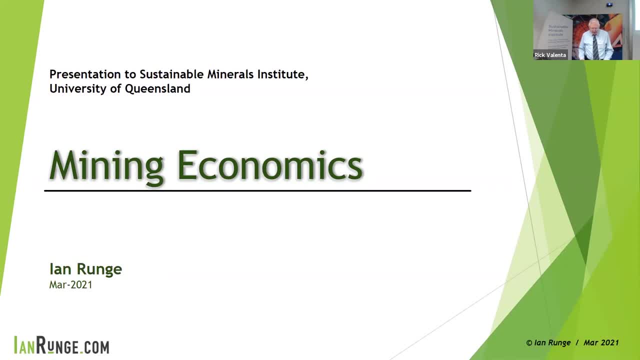 Well, I'm trying to keep my talk informal, but when you have to have it prepared for a webinar, it needs to be a certain amount of structure to it. So get this one right. Oh well, there goes that one. 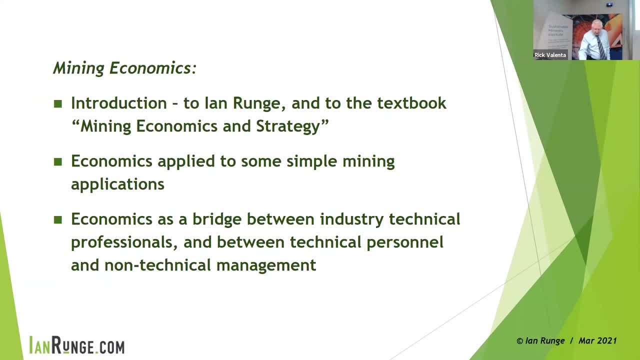 In for next. So I'm going to start, I'm going to introduce myself a little bit and my textbook Mining Economics and Strategy and What's in That. The bulk of my talk will be on a couple of examples of applied economics and alerting you to some of the things that we do now and some of the things that maybe what we do. 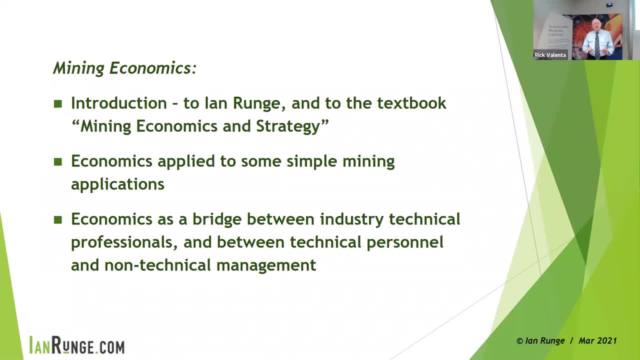 could be done better. And then, at the end, I'm going to talk a little bit about using economics as a bridge between technical people. Well, one you know, say mine, Mining engineers and processing people. that are all between technical people and management of the company. 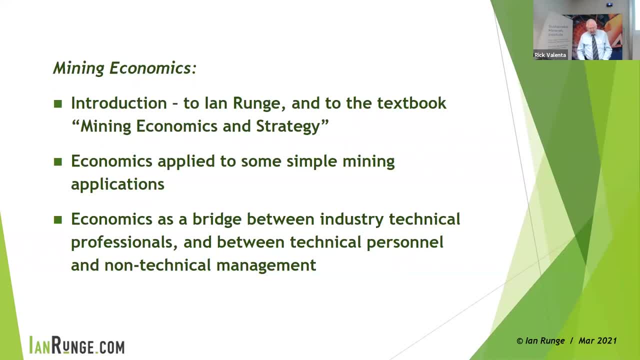 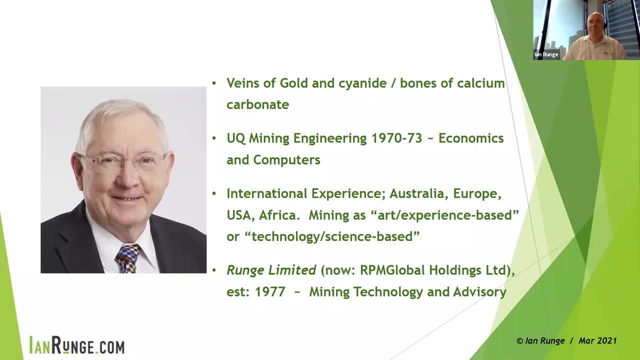 And I'm going to also introduce a couple of examples on how we deal with uncertainty. Well, first of all, let me introduce myself. I was born in Gympie and my father was a metallurgist, And our family was involved in retreating gold tailings using cyanide to recover the gold. 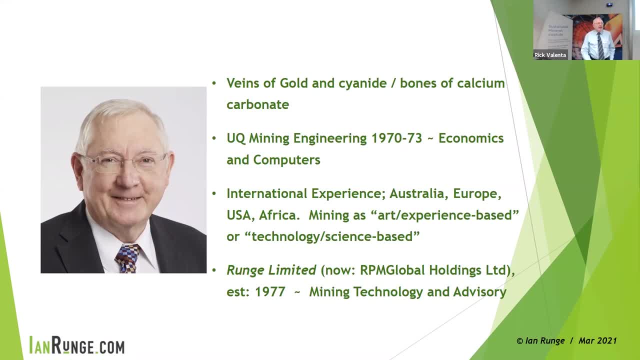 And that was in the 1950s. And as with any retreatment business, the reserves are finite and ours were running out, And until there was a big flood on the Mary River and that finally sealed our fate for that business. And I say our because, but I was only a kid- 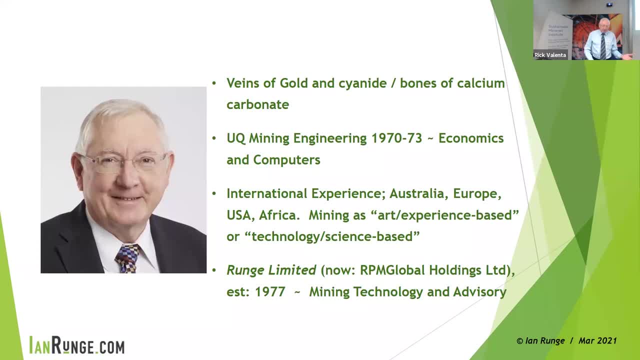 But you know, mining is one of those industries that kind of gets in your blood and your bones And for our gold, Gold, Gold retreatment business We'd been mining our own limestone. So when the gold ran out we were in the limestone business. 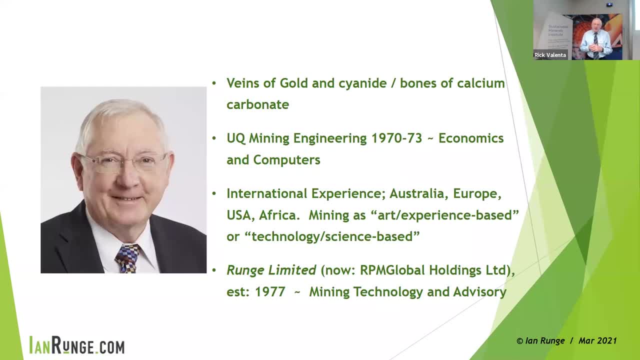 Supplying ground lime for fertilizer and glass manufacturer, Calcined lime for sugar mills and foundries and some hydrated lime. So that's what I did every weekend when I was growing up, You know, charging up the calciner. But although we didn't call it a calciner then, 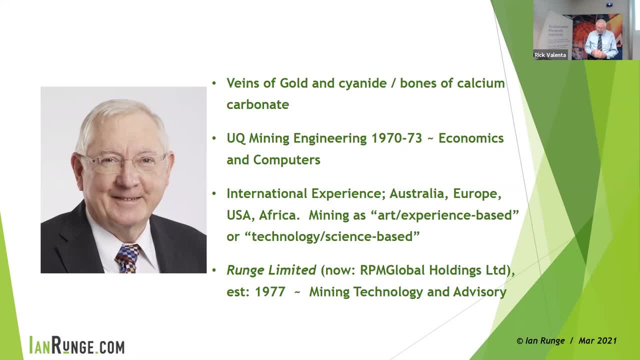 It's just a big vertical Kiln fired by wood- Not exactly carbon neutral, but this was in the 1950s and 60s. I did my undergraduate here at University of Queensland in mining engineering, So I'm a mining engineer. 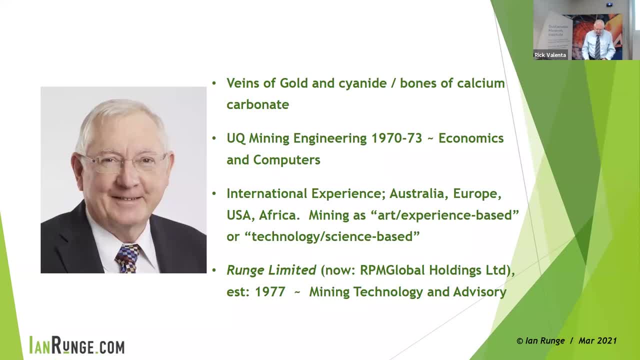 So spoiler warning for you- mineral processing metallurgy people. Later in my talk I've invented a couple of mineral processing examples, So if I haven't got it quite right, you've got to cut me some slack. After graduation I worked at the Siraji mine in central Queensland. 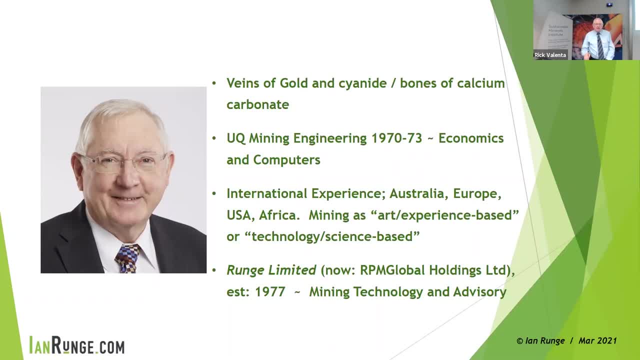 I worked for the coal division for Shell in the Netherlands. Well, there aren't any coal mines in the Netherlands, but we were working on projects in Australia and Indonesia and South Africa. I worked for a mining contractor in the UK called Miller Mining and they had five pits in Yorkshire, Lancashire and Scotland. 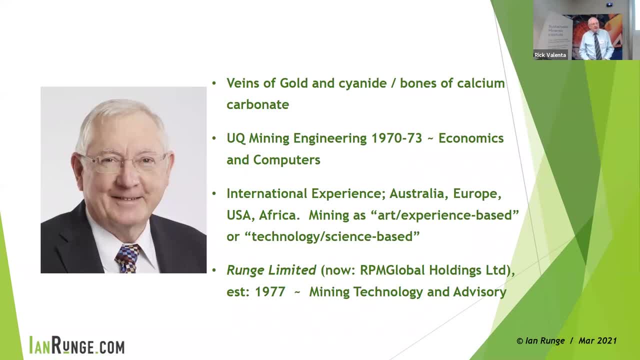 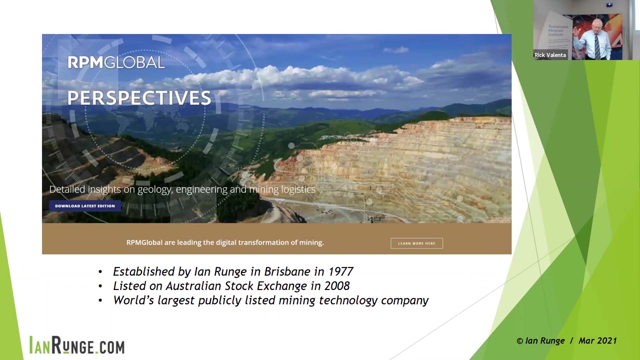 I've always been passionate about using computers To solve mining problems, So I started a company, Rungi Limited, in 1977, focused on computer applications in mining, And the company is now called RPM Global Holdings Limited. And I'm just the R part. 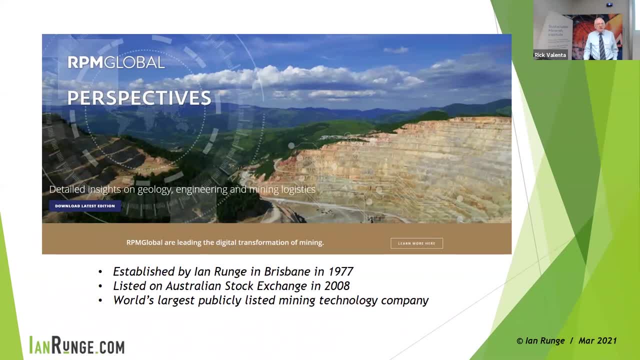 And the business is a mixture of consulting, advisory work and software for mining. But I retired from the board in 2018, after 41 years, and now I'm just an investor, albeit with residual emotional attachment. Well, that's until they do something wrong, and then I'm out of here. 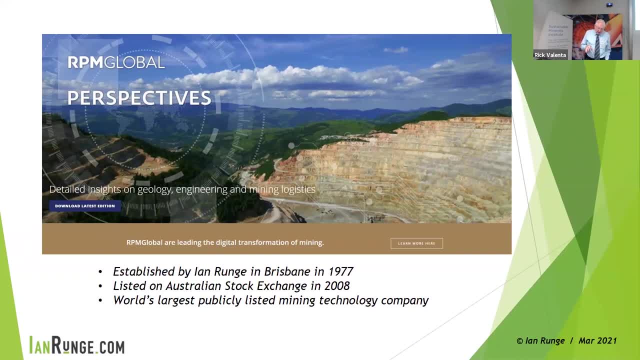 And now I just want to deviate a little bit from my introduction to talk a little bit about writing software- And I'm sure quite a lot of you people are involved in doing exactly that- and particularly simulation software, And why I'm such a supporter of this endeavour, which I think is about the highest technical art form we have in the world today. 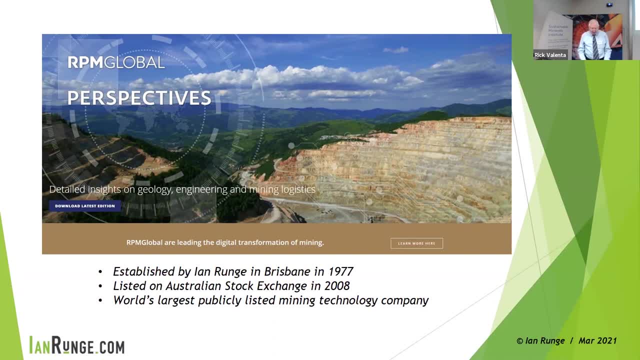 Take a bow, those people doing that. If you try to write a computer program to simulate something like a shovel, truck or drag line- which is what we did, or I'm sure that's the same whether you're simulating comminution or flotation- 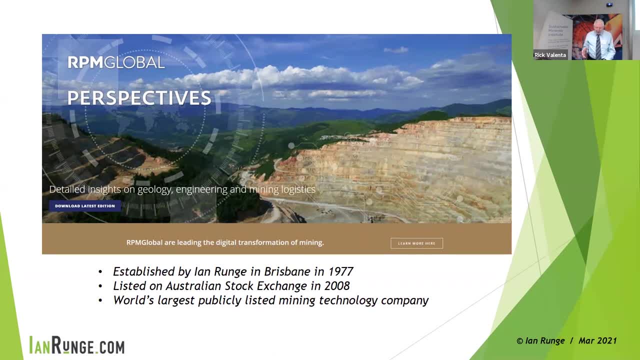 you end up learning so much more about that thing than you ever conceived. The first simulations might work on some narrow set of conditions that you first were looking at, But as soon as you try to apply them into some other set of conditions, it'll fail. 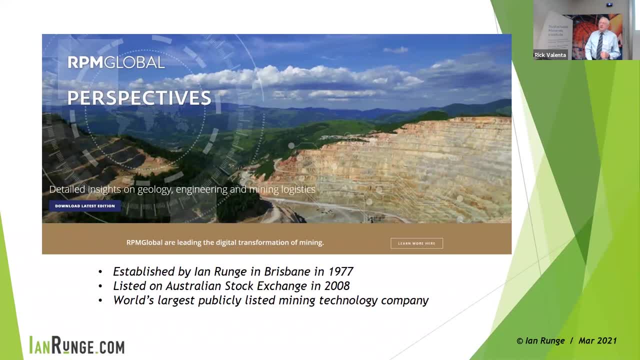 You discover something that you thought you understood was just a narrow subset of some much bigger issue. So you go back to the drawing board, rewrite it, And the next rewrite will expose some other shortcoming in your logic or in some data requirements or something. 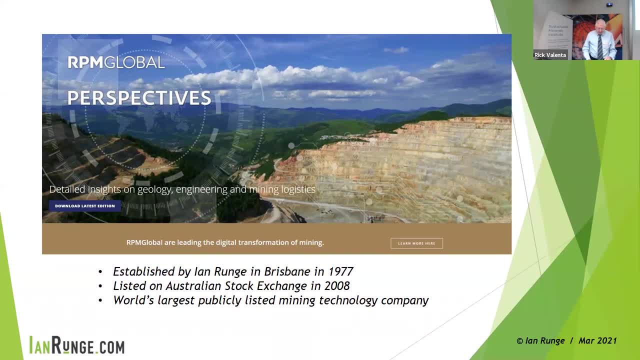 You keep going until you get it right And, as I said, you end up learning much more about that thing than you ever conceived. And that's what was the case with us in the early days of Runge Limited. Our focus was on three main areas. 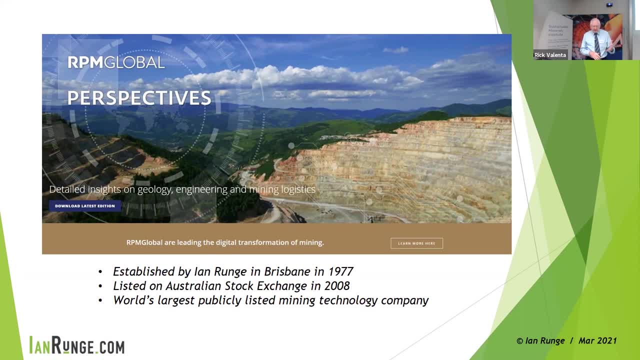 Simulation of mining equipment: trucks, shovels, drag lines. You might have heard. our most notable product out of that time was called Talpac, a truck and loader product. It was a product that was used to do productivity analysis and costing. 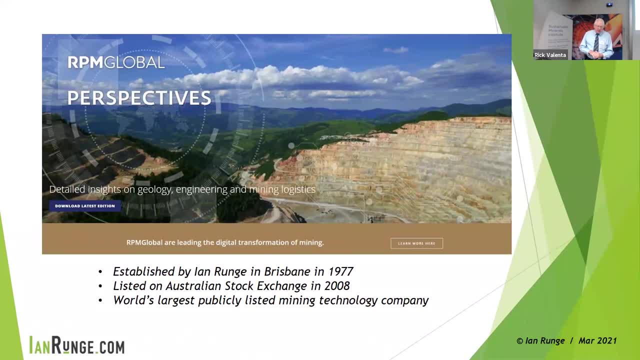 And we've got some variations on that now. Our second area was in mine scheduling And our most notable product there was called Xpac- still is- We've got some variations on that now- called Xact, which is medium term planning, and Xecute, which is short term planning. 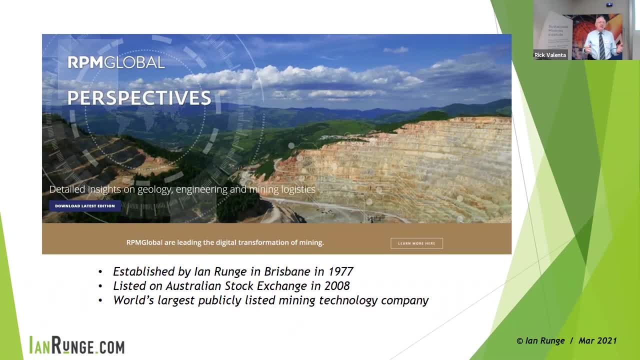 And the third area was financial modelling, particularly for budgeting, equipment replacement analysis and economics, And that product's called Xerus. The E-R-A-S is equipment replacement analysis originally. Now, as a result of being so heavily engaged in this simulation and modelling, 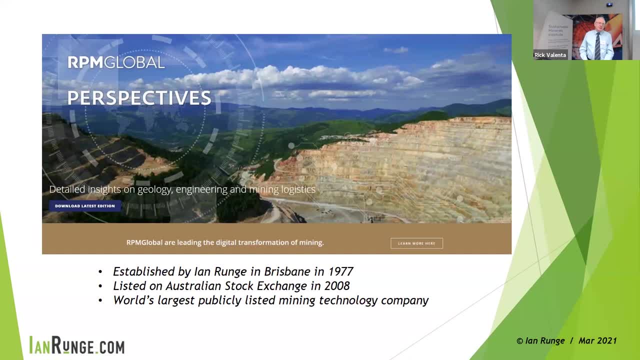 we ended up knowing more about these things than just about anybody. So in 1984, I started presenting professional development courses in these fields, including mine: economics. It was a way to sell our software, software and consulting services, for sure. But it was also a way- or at least my attempt. 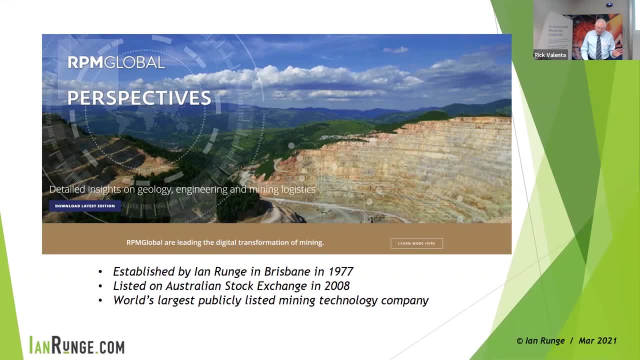 to move the industry away from the old rules of thumb way of making choices into one based on science, technology and economics- And you'll hear that term rules of thumb quite a bit over the rest of my talk, Which brings me back to economics. 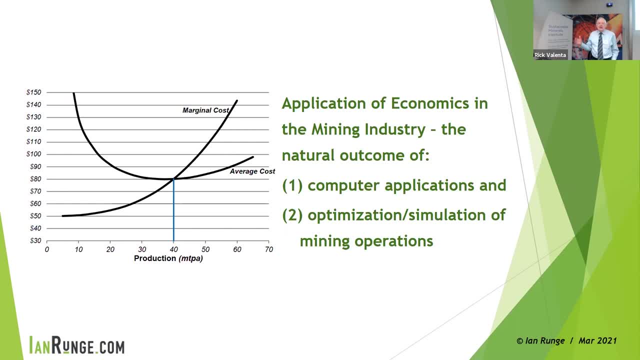 When you analyse something, simulate something, what are you trying to achieve? What's your objective function? Is it optimising productivity or optimising yield? Well, optimising productivity or yield will only get you halfway there. You know how can you compare, say: 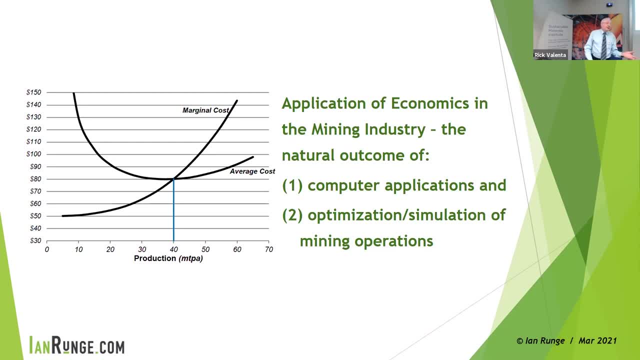 a 15 cubic metre loader with 130 tonne trucks against a 25 cubic metre loader in its fleet of 230 tonne trucks. The two systems have totally different capital and operating costs. If you keep following that logic, it'll invariably lead you to conclude that your objective function. 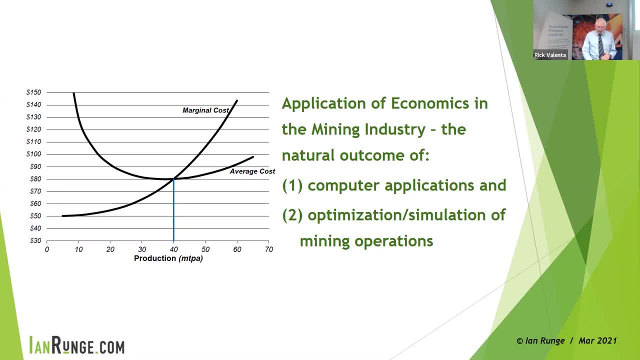 is actually an economic one, an economic alternative. That's what the company wants. In the case of trucks and loaders, what the company really wants is the cheapest way to move the dirt. They don't care what your truck match is or how many passes it takes to fill a truck. 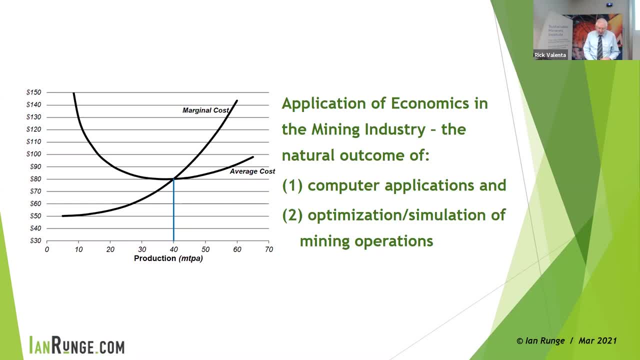 All they want is the cheapest way to move the dirt Now in a processing plant. usually people are after maximising the yield, And actually that's a pretty good proxy for economics, because maximum yield probably equates to maximum revenue. But what about the processing cost? 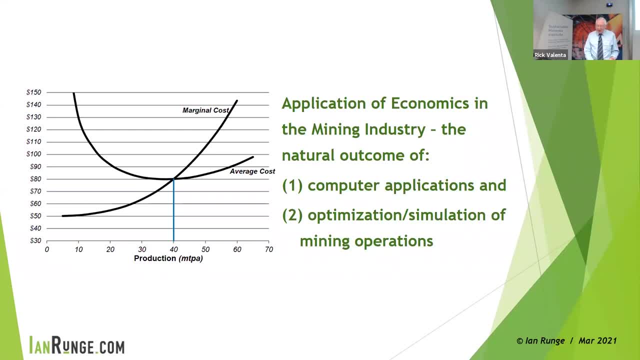 Froth flotation might give you the highest yield, but if a simple jig will give you nearly as good a yield and have much lower operating and capital, then that might be a more economical alternative. In the pre-computer days many of these things were virtually impossible to calculate. 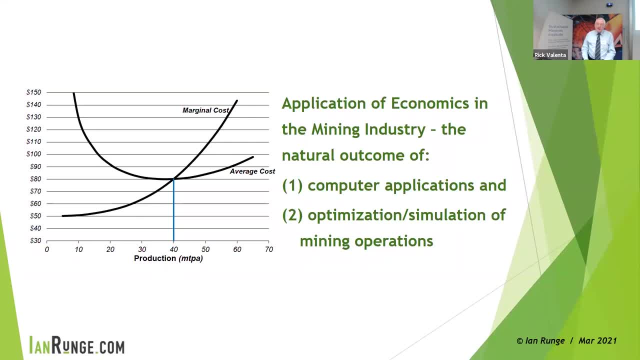 We had to use rules of thumb as a proxy for economics. Now that's not the case. So this is the foundation for my move from being primarily a technical boffin to a different kind of boffin: economics: focused Applied economics. 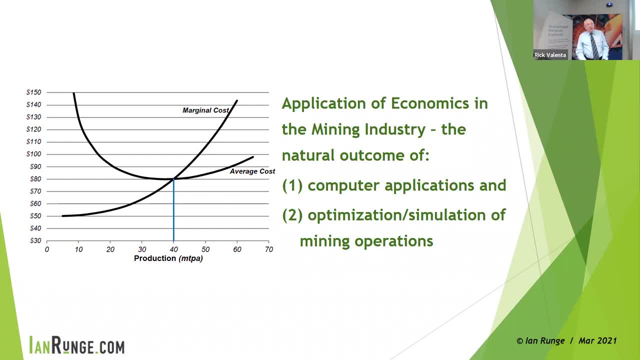 By the early 1990s, having been through several industry booms and busts, I was disillusioned with the application of economics in the industry. Actually, on the technical side, the production people, I think we'd made some good progress. 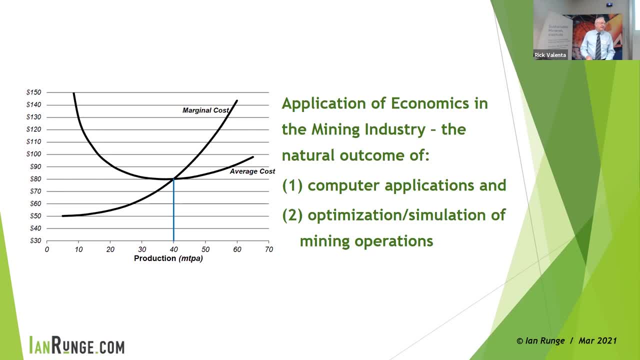 But on the management side of the industry their report card was a C- Now I was going to talk a bit about that, but it got to be pretty negative and I don't like to finish my talks on negative. so you can ask me the questions later. 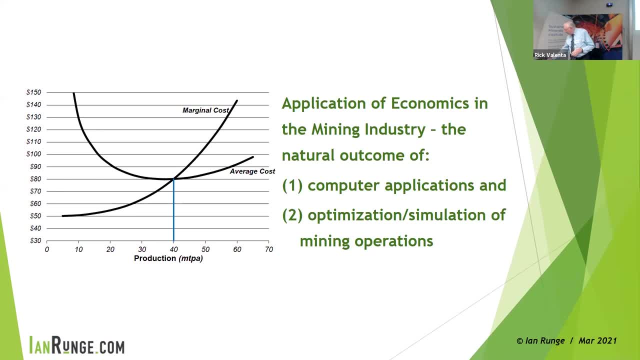 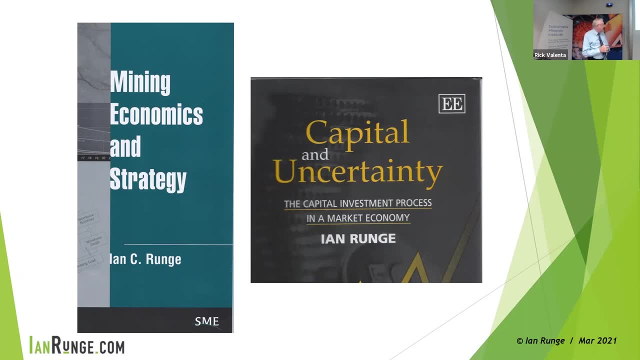 Anyway, to cut a long story short, in 1993, I was at age 40. I took four years off and completed a PhD in economics, and then sat down and wrote my book Mining Economics and Strategy, which was published in 1998.. 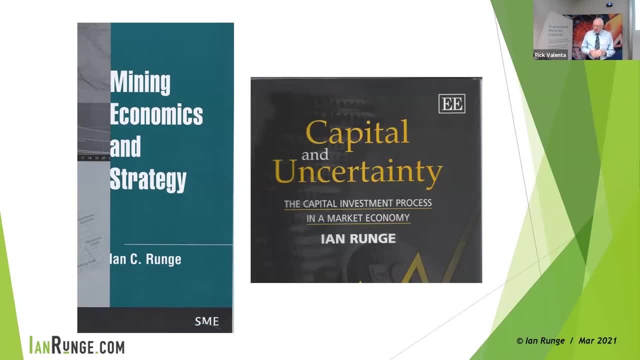 And then another two years later. I took four years to write my book Capital Uncertainty, which was published in the year 2000.. Now, Capital Uncertainty, you've probably not heard about. It's not a textbook, It's an economics reference book. 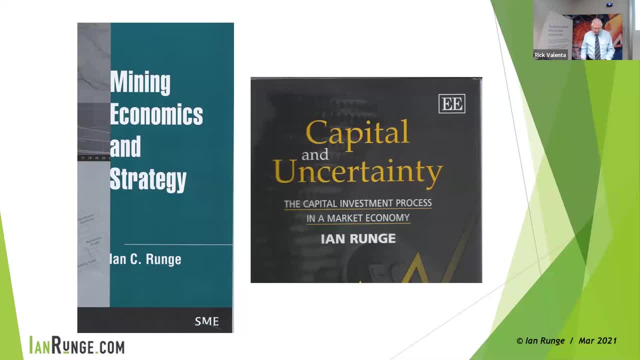 on rational decision making for choices under uncertainty, particularly pertaining to large capital investment decisions such as the decision to start up a mine or not, Which brings me to where we are today. My mining economics book was essentially made up from two professional courses. 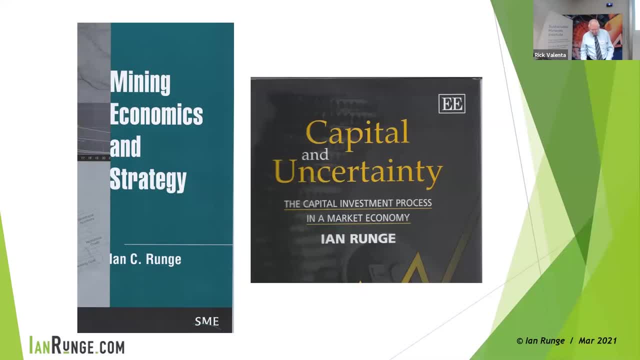 that I had been presenting. The text was quite coal focused, quite open pit mining focused and directed mainly at mining engineers, not geologists or process engineers, And over the time the book has become the biggest selling textbook that the SME publish. 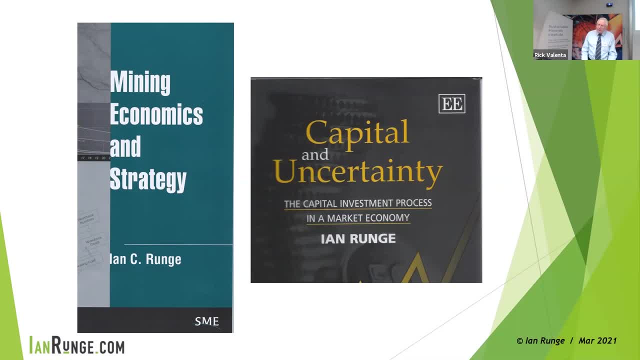 but it's also found its way onto the desks of a lot of people who were never really in my target audience, such as mine accountants, A few mineral processing engineers, suppliers to the industry and people in government regulation wanting to know a little bit about economics. 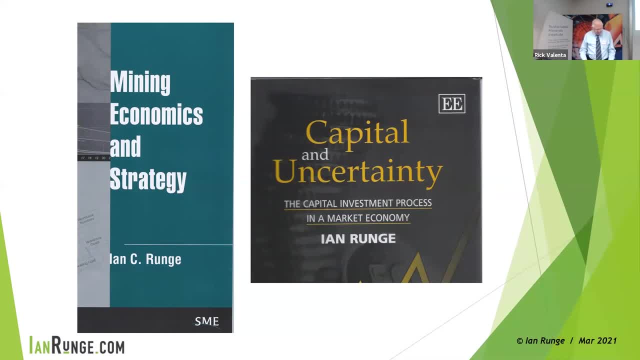 of the mining industry And I figured that's a lucrative area to work on because I don't know how much they know right now. So anything we can do has got to be a help. So I'm in the process of rewriting it with specific introductory chapters. 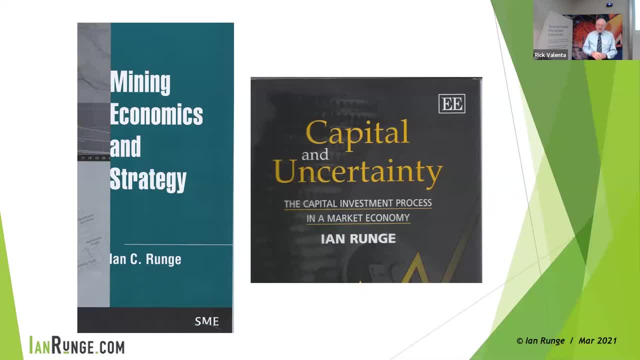 at people who don't actually have a technical background in the industry, as well as examples from a wider cross section of the industry- underground mining, more metalliferous examples, mineral processing- And I'll be also including some of my text or revised text from my Capital and Uncertainty book. 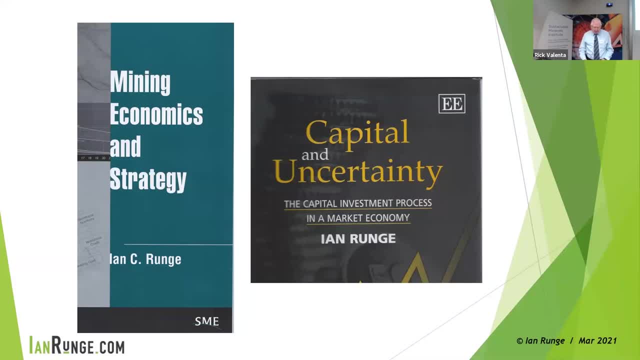 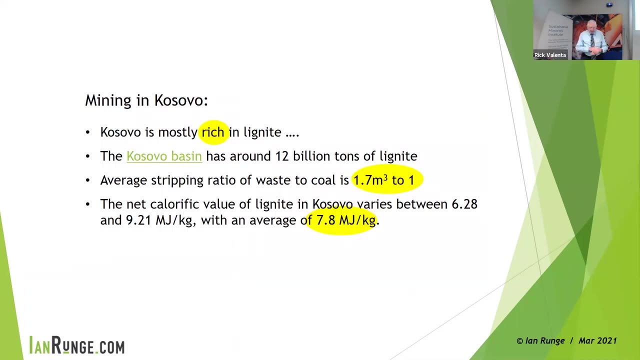 involving mining decisions where there's risk. So after today's talk, I hope to get some additional examples from your areas to mix with my examples from the book. Now that all sounded like a long introduction, So let me take you through a first really simple example. 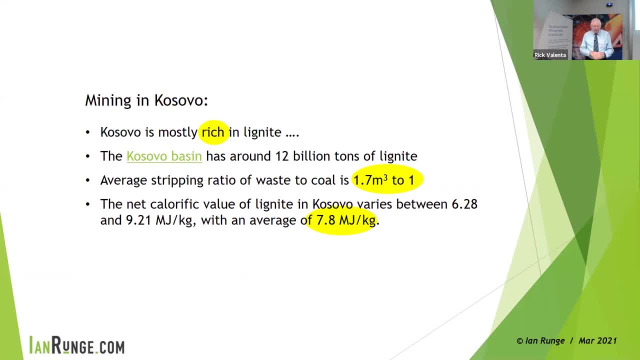 illustrating the importance of applied economics to all of our technical decision making. I was scanning Wikipedia last week and came across this entry on Kosovo. I don't know anything about Kosovo. It says that Kosovo is rich in lignite implied by their large reserves. 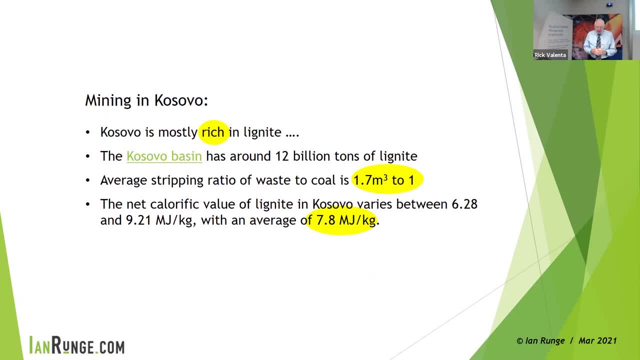 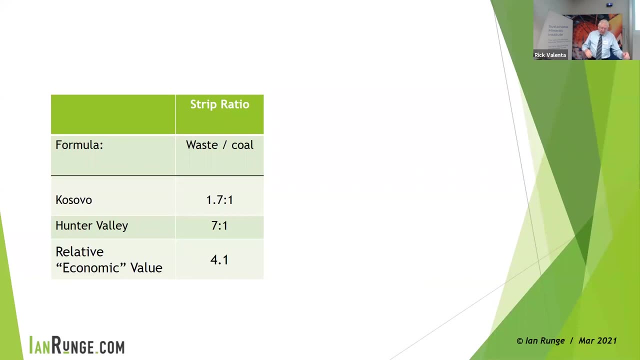 and presumably low stripping ratio of only 1% or 1.7 to 1.. What does that mean? In the Hunter Valley the stripping ratio is typically around 7 to 1.. So you know we're using stripping ratio. 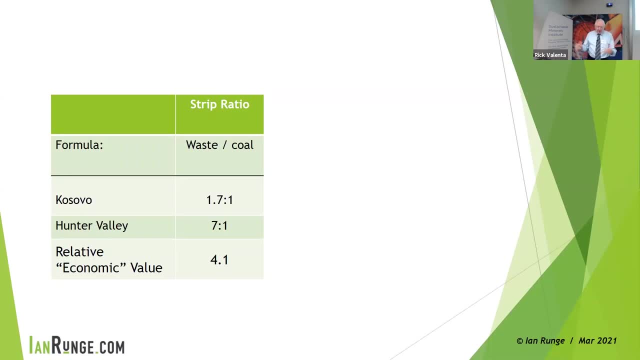 as a proxy for economics, And from this you'd be inclined to think that the Hunter Valley coal is sort of economically worse or more costly to mine by a factor of 4.1 to 1.. But is it Well when you're mining? 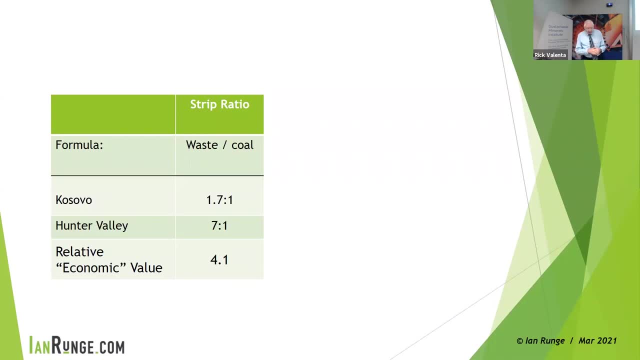 you not only have to mine the waste, but you have to mine the coal as well, And there's a cost to that, And a ton of coal probably costs as much to mine as about a cubic metre of waste. So slightly better if you're going to use a primitive indicator. 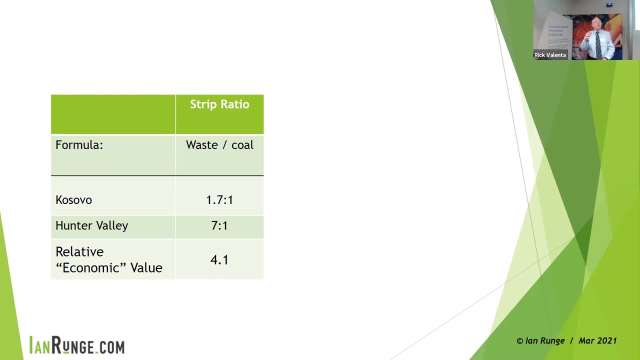 like strip ratio. a slightly better one would be the waste plus the coal divided by coal. So, and in which case you have got 2.7 in Kosovo and 8 to 1 in the Hunter Valley, And so Kosovo's only on that measure. 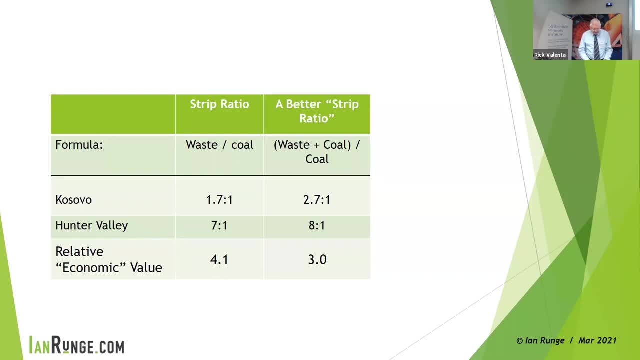 three times better than the Hunter Valley. But wait. the calorific value of the Hunter Valley coal is 7.8 megajoules per kilogram. Hunter Valley is three times that much And after all, it's those megajoules we're really after. 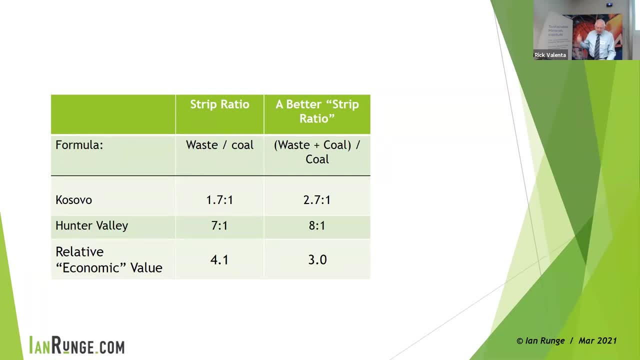 not the tonnes. So if we have the waste plus coal divided by megajoules, we find that on a calorific value basis, Kosovo tonnes are no better than the Hunter Valley, And if there's transportation involved, those Kosovo tonnes are even more disadvantaged. 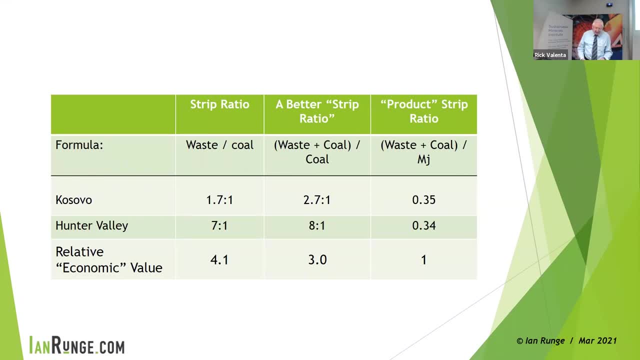 because they are three times more expensive to transport on a megajoule basis than is the Hunter Valley coal. So we use strip ratio as a proxy for economics because it's easy to calculate, But like many rules of thumb that are a hangover from the past, 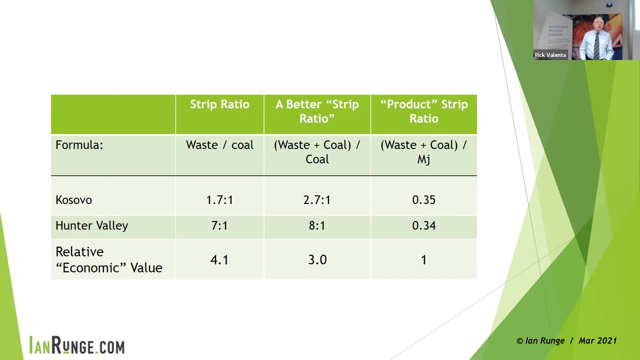 the imprecision of the rule is no longer tolerable considering the ease of calculation of the real thing. I wrote a paper in 1988 for a conference in Canada. it said: strip ratio, an outdated indicator of economic value. Don't get me wrong. 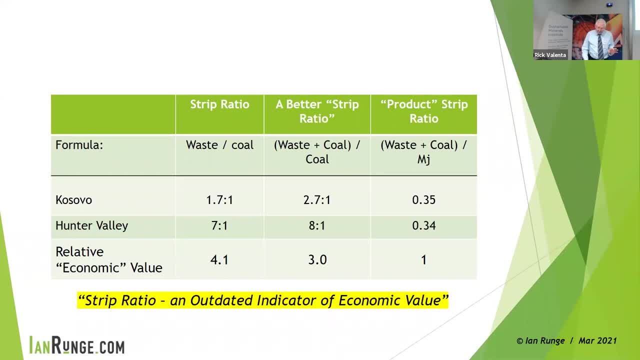 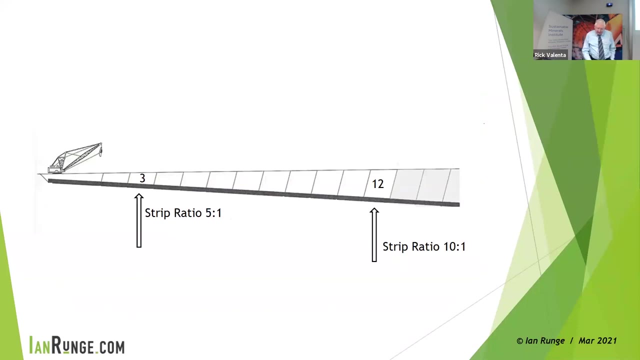 we do need rules of thumb from time to time, but we need to be satisfied that they are a good proxy for the real thing that we're after. If the mine is simple like this single seam dragline mine, then strip 12 will have a higher stripping ratio. 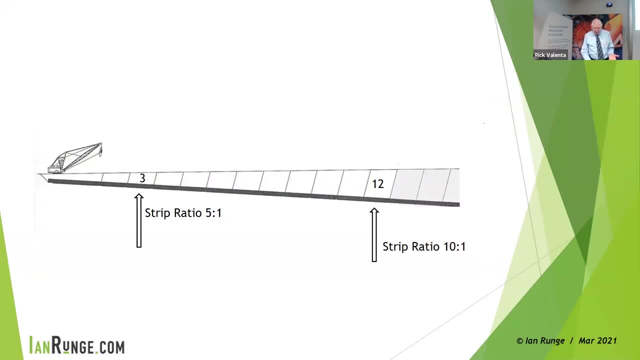 than strip 3, and you can be confident that strip 12 is less economic than strip 3.. Fair enough, The rule of thumb stripping ratio is a reasonable indicator, or at least a relative indicator. Well, in fact it's not even that. 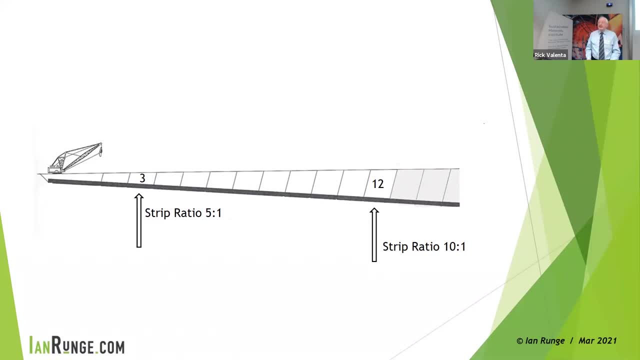 It's a fair rank ordering indicator of economic value. We persist in using outdated rules of thumb such as stripping ratio because, well, we don't always have the time to sit down and work out the correct comparative number, Well, we might be lazy. 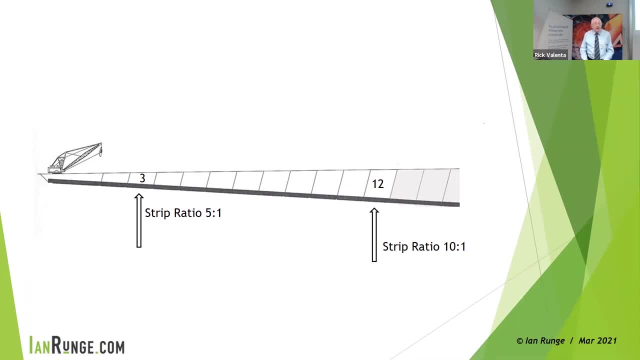 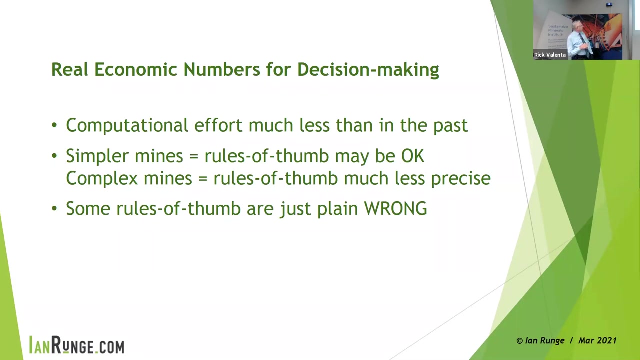 Or maybe we love doing technical calculations but we don't like doing economics. Or maybe we don't know how to calculate the correct economic number to use for our assessments. So this is actually what my mining economics book is all about. It sets out the tools for technical people. 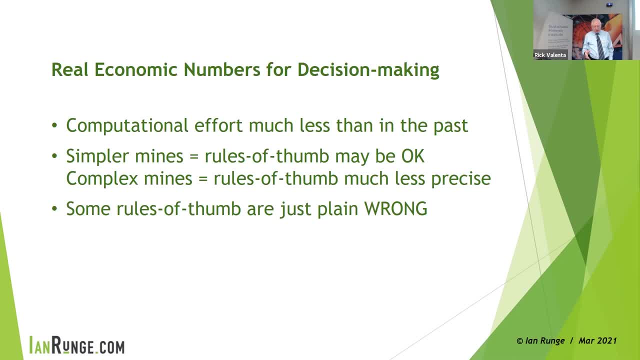 to apply good economics to each choice we make. And I'm talking economics 101 economics, not PhD economics. It's dead straightforward. We should be doing it. Firstly, the computational effort to work out the economics is much less now than it was in the past. 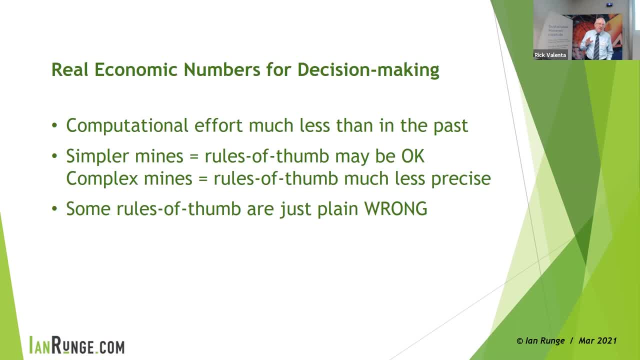 Secondly, mines in the past were invariably simpler, like that simple dragline mine. so some short form rule of thumb was arguably not so imprecise compared to the real economic number if we had have calculated it. That's less so the case today. 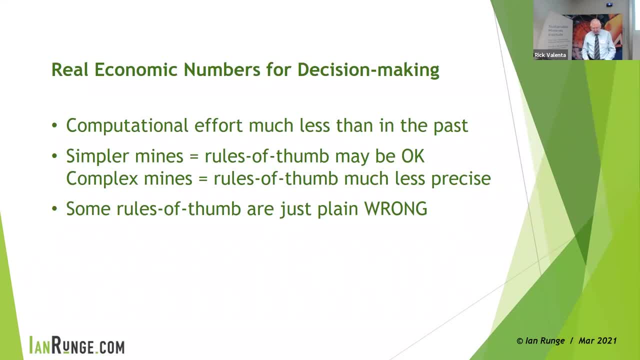 And thirdly, some of these rules of thumb that we continue to use are just plain wrong. So let's move on to another simple mine case study. Simple in the sense that it's easy to understand, but an illustration of how, if we aren't on top of the economics- 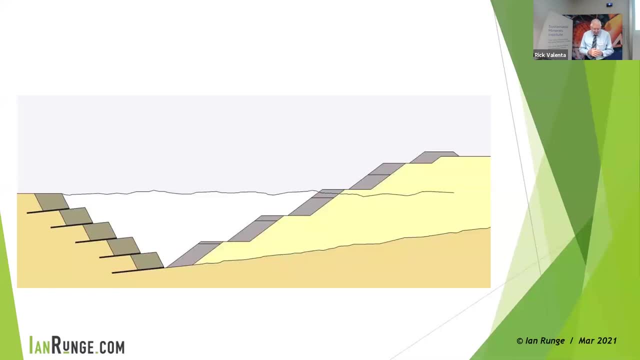 we can get it quite wrong. So this is a cross section of a multi-scene coal mine, typical of those in the Hunter Valley. Mining is straightforward: You excavate the waste from the left-hand side and dump it on the mined out pit. 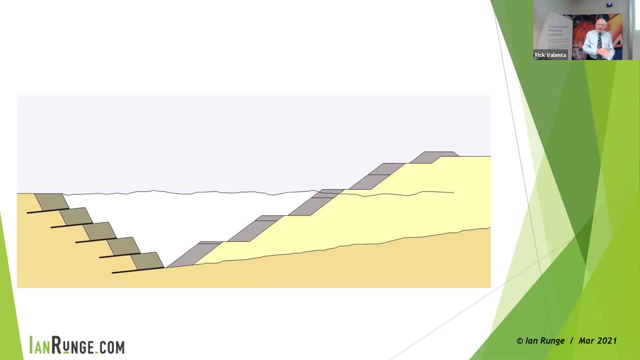 on the right-hand side, advancing down, dip one strip at a time and rehabilitating the ground behind you as you go. Now this example has a 10 to 1 stripping ratio for all five scenes. If you had a choice, would you mine all five scenes? 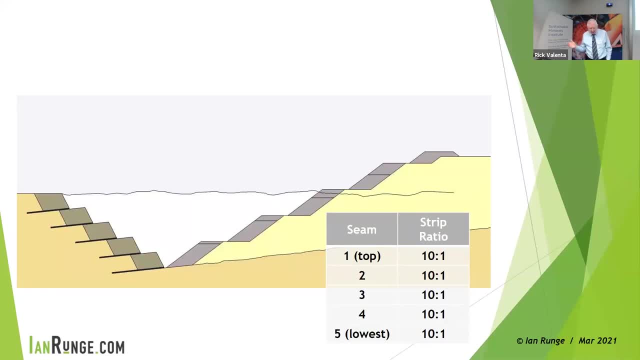 Or is there scope to maybe only mine the upper two scenes, perhaps leaving the rest for later underground mining? Well, using the strip ratio calculation, there's no way to differentiate between these seams, But, as I've already pointed out, strip ratio is only a poor indicator. 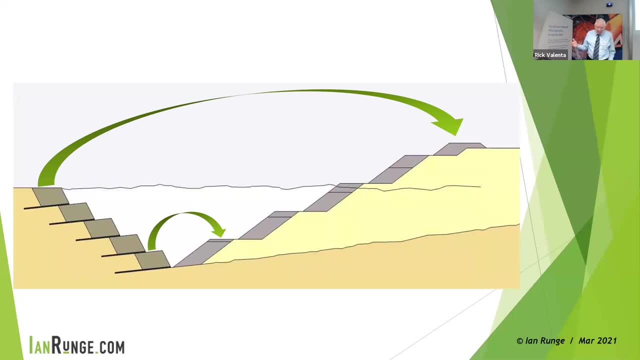 of economic value. For example, the waste above the lowest seam only has to be dumped in the bottom of the adjacent mined out pit. You might even be able to use a drag line. It's going to be cheap. It's going to be much lower cost waste. 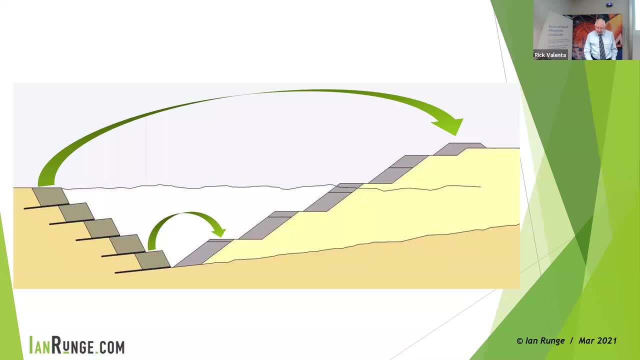 than the ones you're moving to uncover the top seam, which has to be hauled a much greater distance across the pit and raised a much greater height. So let's start thinking. how can we apply some economics to these calculations If we had a good accounting system? 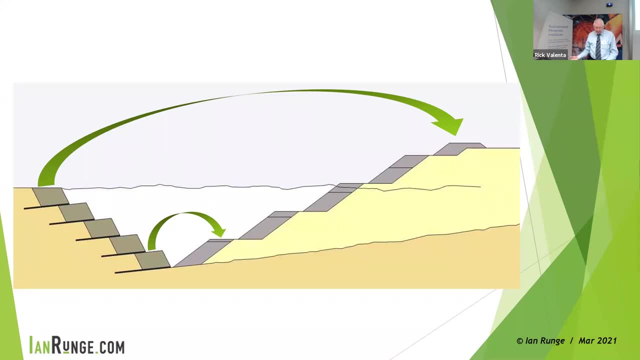 the tracked waste moved by seam horizon. I could work out the cost, or it should tell us the cost- on a seam by seam basis. Well, here's what it would look like. It would show that the coal from the lowest seam is the lowest cost to mine. 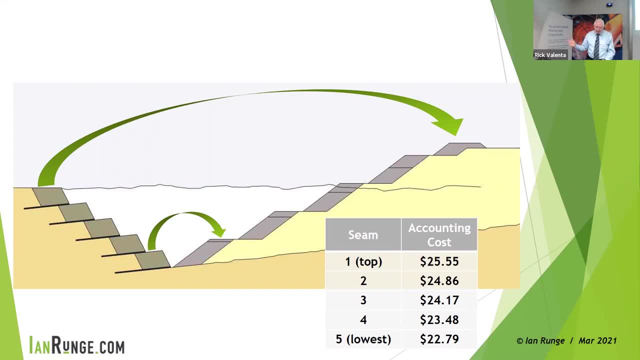 Is that a reliable number? Well, it comes from your accounting system, so it should be, But I think, as everyone recognises, the numbers from an accounting system are seldom useful for planning purposes. To make mine, any planning decision, any forward-looking decision, 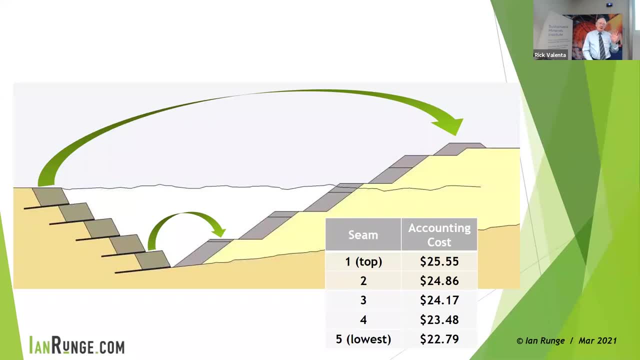 your choices have to be based on one plan that you might do from now and into the future, compared to some other plan that you might do. And once you've chosen and implemented one such plan, you'll have the accounting data for that plan, but you'll never have accounting data. 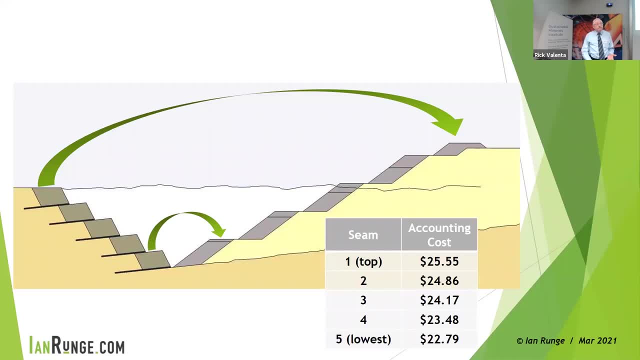 for the alternative plan that you never did implement. Costs for an economist are something that informs decision-making. They're not some historical thing incurred, And if I want to Imagine you're running this, mine or maybe an accountant in your company is insisting you've got to cut some costs. 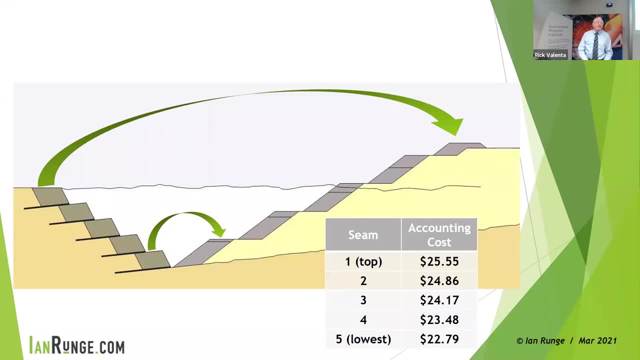 in your operation. He could look at your accounting figures and if I want to have a cheap shot at it, Any accountants here? Okay, that's good, If I want to have a cheap shot at accountants. I can imagine someone saying: 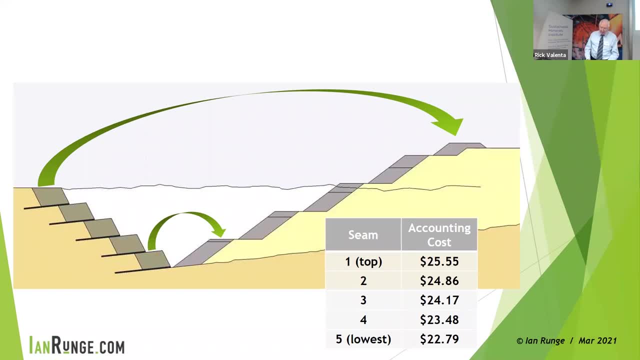 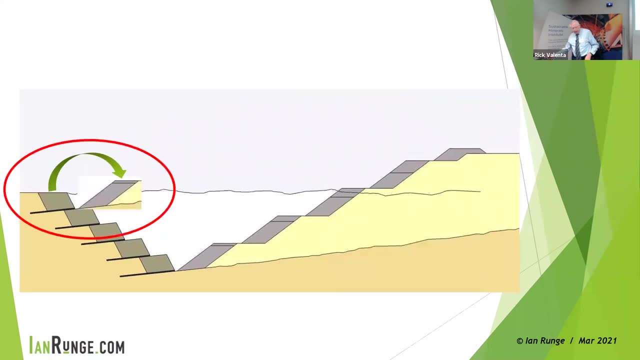 well, we could significantly improve the economics of this mine by only mining the lower seam, And it's easy to see the shortcoming here. If we only mined the upper seam, we wouldn't have to haul that waste all the way to the other side of that big pit. 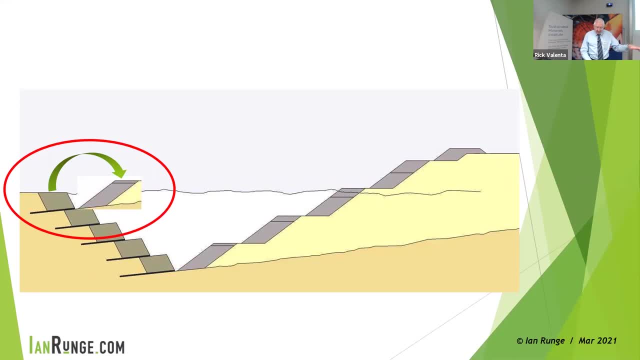 We'd be dumping it in the pit right adjacent because that's where we'd be. Its cost would be much lower than what our accounting system shows our costs to be here, And that's the cost that we need to think about as applying to that upper seam. 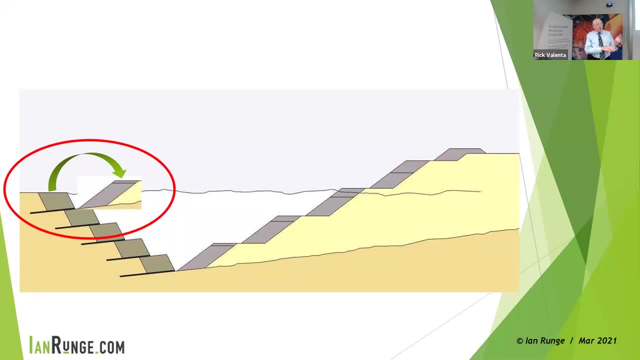 that has to inform our choice. for that We can work out the real cost of mining a second seam. the same way, We have to plan the entire mine as a two-seam mine. subtract from that total cost, the total cost of a mine plan. 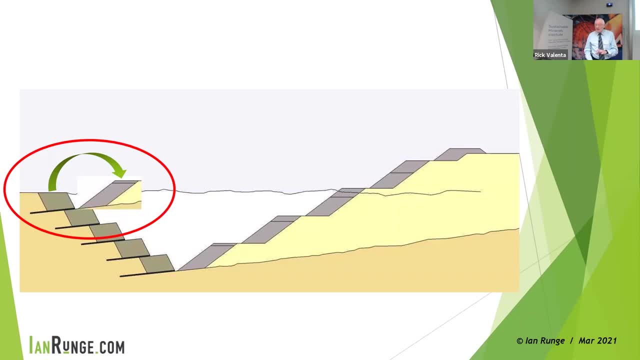 predicated on just the uppermost seam And the difference is the real cost of mining seam number two, That is, the marginal cost, is the change in total cost and it's the marginal cost that we must use in deciding whether to mine that second seam or not. 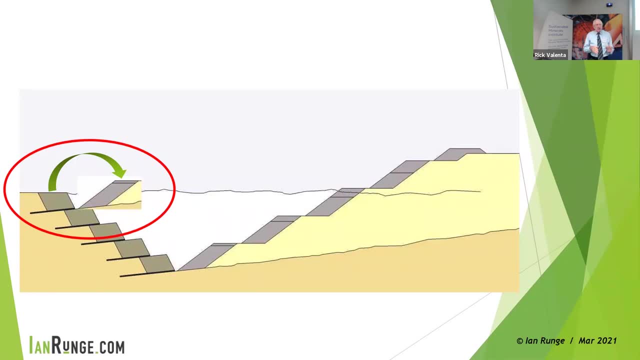 And we must continue in that way for all of the seams. So this concept of marginal cost is vital for any economic analysis. Understanding marginal cost is the key to deciding just about anything, whether it's the various mining alternatives or the split between fines and course. 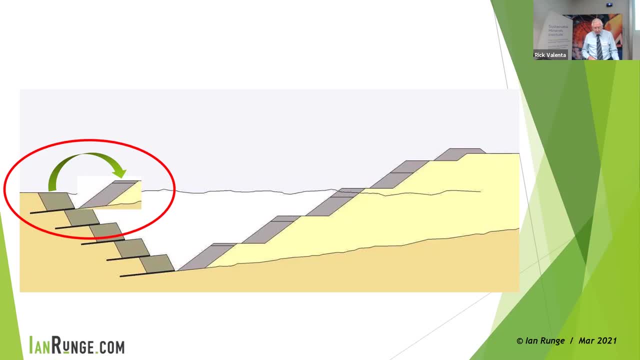 in a processing plant or anything else. Here's the key, though: The marginal cost can't be measured, You can't get it from your accounting system. It has to be calculated. And the great news, finally, we have computer power enough to do these calculations. 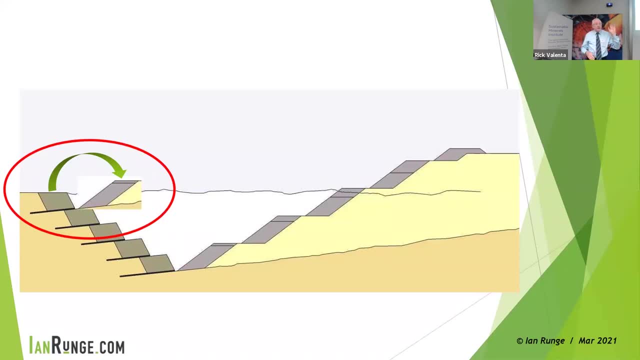 which is what I've done here. I've considered five different scenarios: a one-seam mine, a two-seam mine, a three-up to five-seam mine. I calculated the total cost for each alternative and I determined the marginal cost. 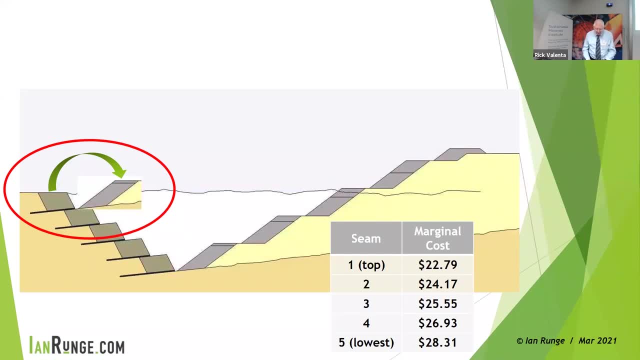 being the change in total cost between each of those alternatives, And the results, as you would expect, show that the top seam is indeed the cheapest to mine. Indeed, it's 19% cheaper to mine than the lower seam, whereas the accounting system suggested. 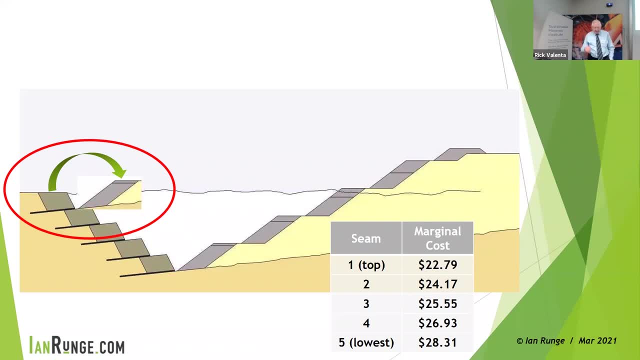 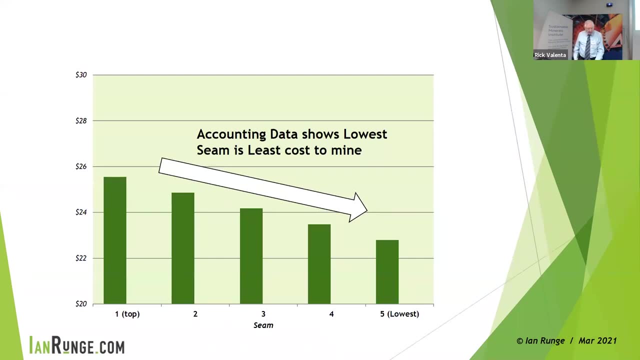 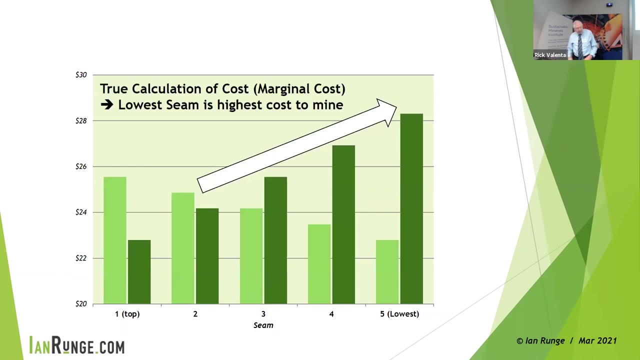 it was 12% more expensive than the lower seam. So we have five seams with the same strip ratio based on reliable accounting data. Mining costs decline as we go deeper, But as a guide for mine design, that's a complete bum steer. 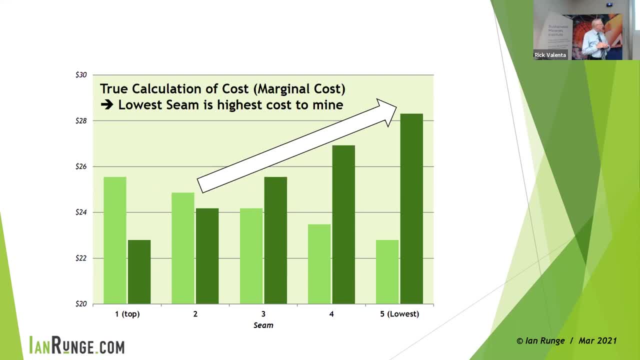 The cost, the marginal cost, increases as we go deeper. This is a really simple example, but I'm sure you can see how, if you look at the figures, calculation of these marginal costs is almost impossible. What if the value of coal characteristics? 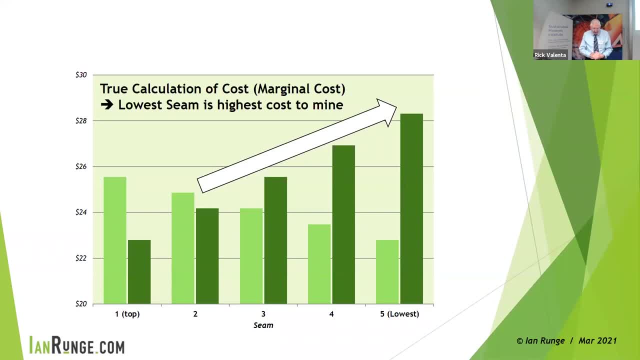 of those seams were different. They will be. Maybe some of them were coking coal and some thermal coal. Do you think it might impact the design of your processing plant if some mining guy stuffs it up here and you haven't got figures there? 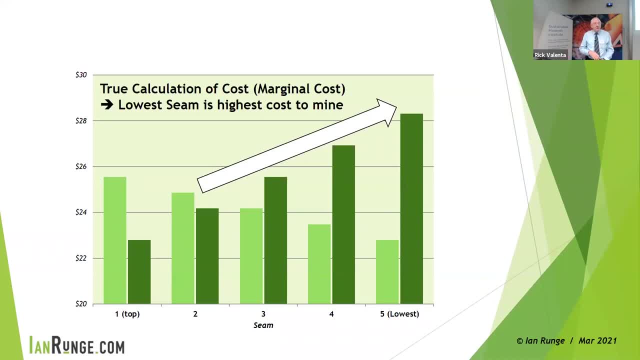 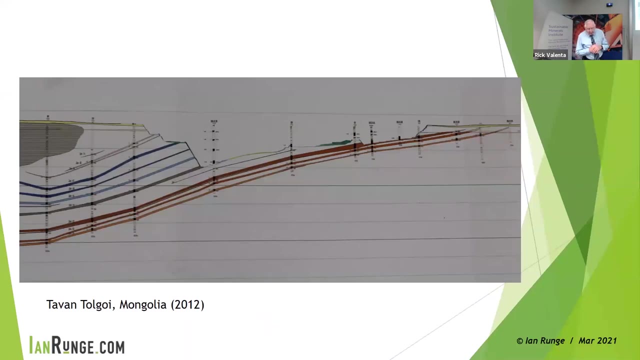 and you've got to design the plant for one kind of coal or the other. It makes it hard to change the plant afterwards, when you've built the plant. How might this look in the real world? Here's actually a cross-section for anyone who recognises this. 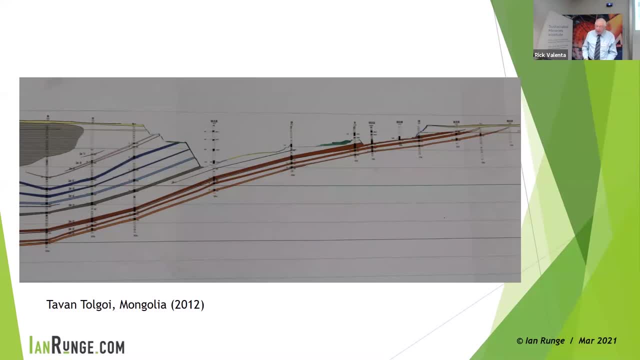 It's from Tavan Tolgoi in Mongolia. The plant there is designed by Siegmund. Does that look a little familiar to that last diagram I just had? Well, in this case the target seam was one in the middle of the sequence. 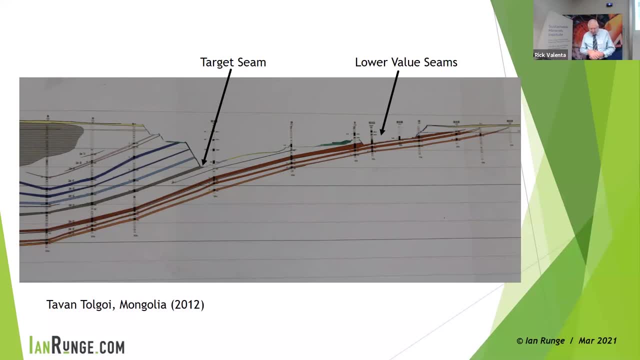 I think it was coking coal- Whereas the lower seams were less valuable. Of course, not mining these lower seams on the way through meant that all the waste had to be hauled out of the pit, and that adds some cost, But that's a story for another day. 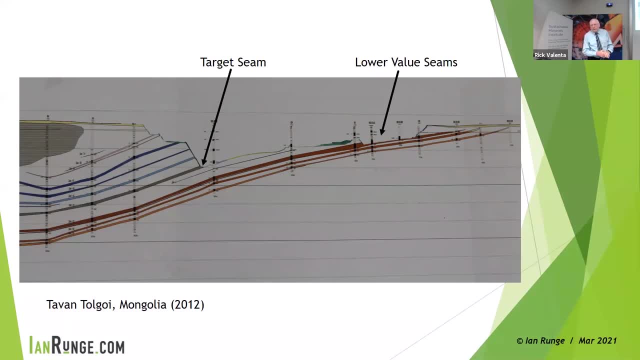 So what I want you to draw out from this example and this sort of concluding the main part of my presentation and I hope gives you a flavour of what economics can do for us and how it can make a huge difference if what we're doing now 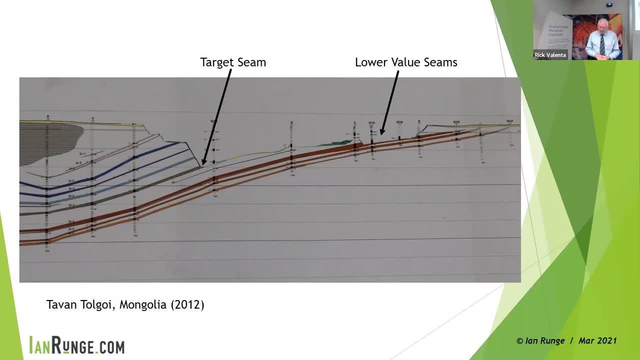 is old rules of thumb that haven't been tested, And so that's two takeaways from this, I think. first of all, rules of thumb: No matter what they are, you must put them on trial for their life. Many of them are outdated. 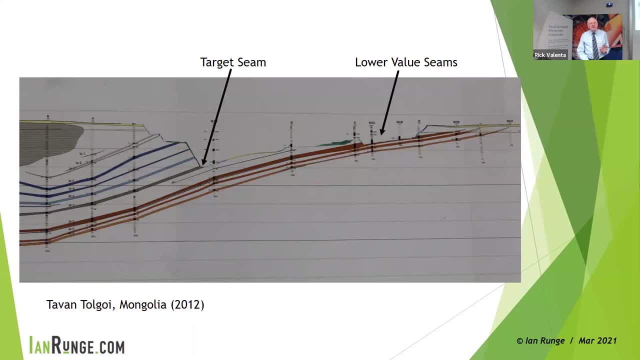 Some of them are just plain wrong, And even the ones that are still relatively good can probably be improved with small computational effort And marginal cost. My mining economics and strategy book is full of marginal cost examples, and my new version will have even more. 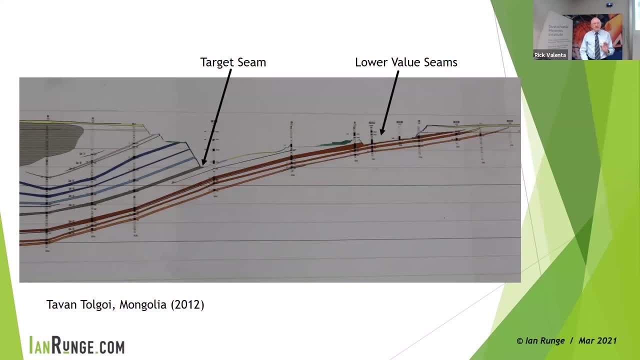 The takeaway from this is: you can't measure marginal cost, You have to calculate it. This marginal cost idea is important, And it's economics 101.. Mind you, I think a lot of economics schools probably don't address this as much as they should. 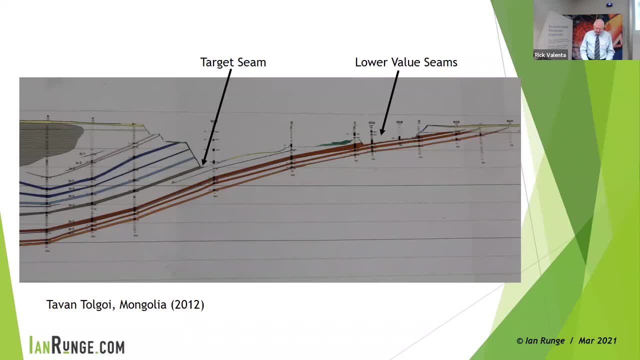 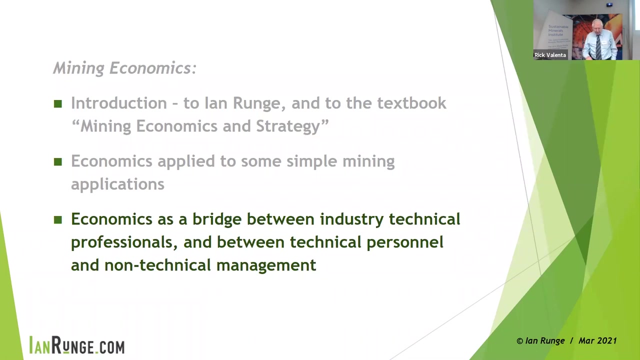 So if this is new to you, then please take it on board. Don't pass go until you've collected your $200 worth of marginal cost. Well, with increasing complexity in mining comes increasing value in better interaction between different technical professionals and between technical professionals. 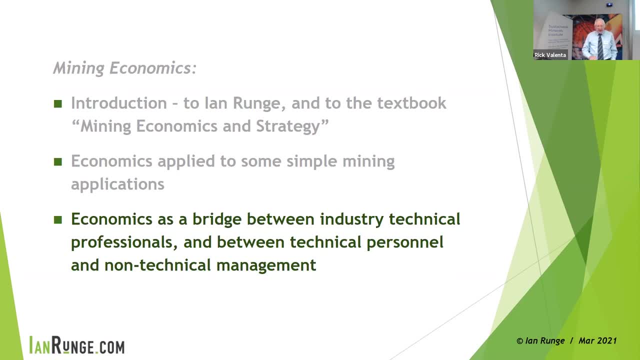 and management personnel And economics provides a unifying tool for cross-disciplined approaches to achieve these outcomes. So here's an example: The interface between mining production people and processing plant personnel- Mining. I don't want to give away a dirty secret here. 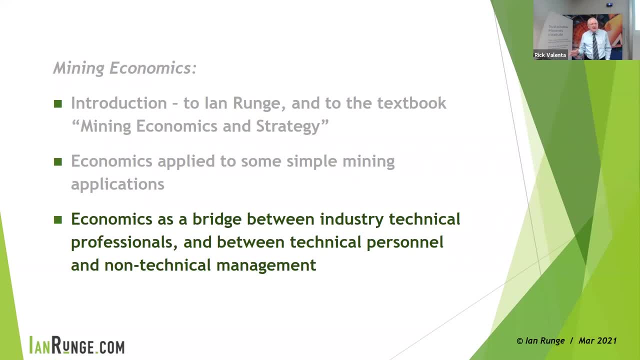 but mining production personnel. classically, we can solve dilution and contamination problems easily just by sending more diluted and contaminated ore to the processing plant. I've heard it multiple times from mining production people: Hey, that's what we've got, a processing plant for. 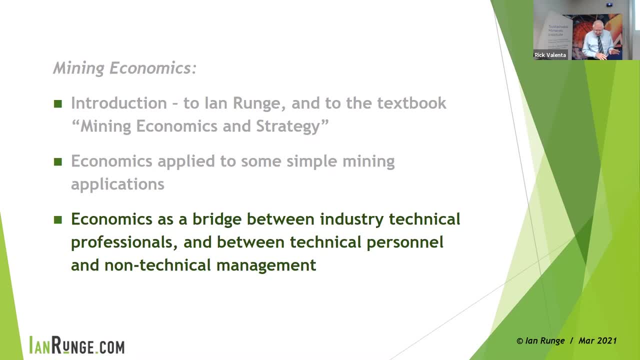 Yet a saving in mining cost might result in a much higher cost in the processing. If the processing plant is not designed to handle the feed characteristics, then the throughput might be reduced. The cost of processing the dilution and contamination might be significant or it might not. 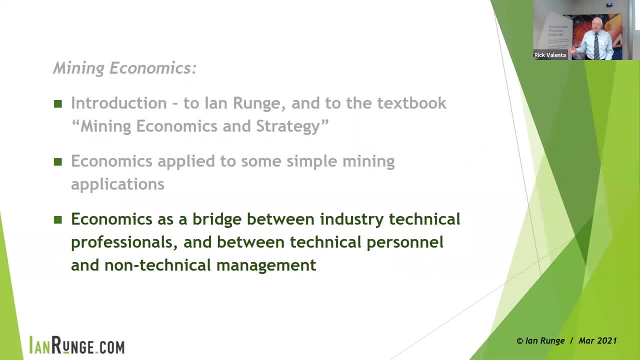 But if the throughput is reduced because of the dilution and contamination, the lost revenue might be many times this. If the processing plant is designed in the first place to handle the different feed characteristics, then this will be a higher capital cost for sure. 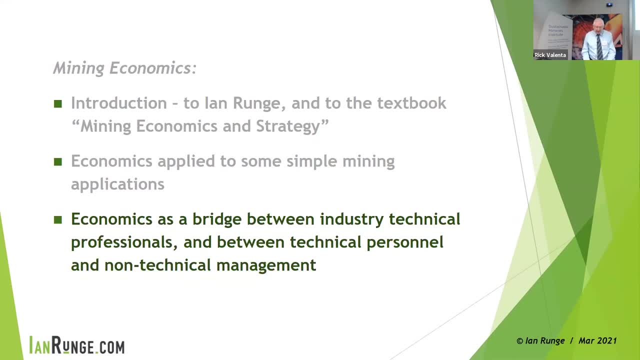 But how significant is this in the overall economics? The impact of the higher initial capital costs may well be less than the additional mining costs of trying to reduce contamination at the mine face, particularly if the mine face is underground in the dark and very constrained. 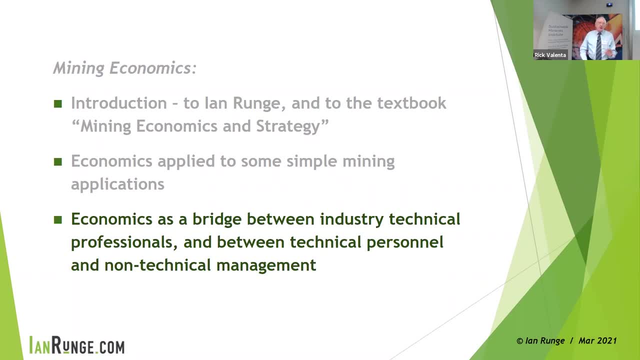 One thing's for sure: a heated argument between the mine manager and the processing plant manager at the daily production meeting won't solve the problem. Economics can, And I'll wrap up with just a couple of examples, I think, of what I'm looking for. 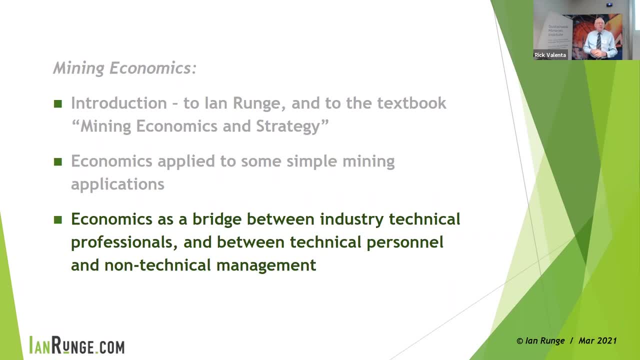 I'm not going to sort of give you anything definitive here, but I want to float a few ideas, some of which will be in my new book. But if there are issues that you're wrestling with, then on my emails, at my website or on there, send me an email. 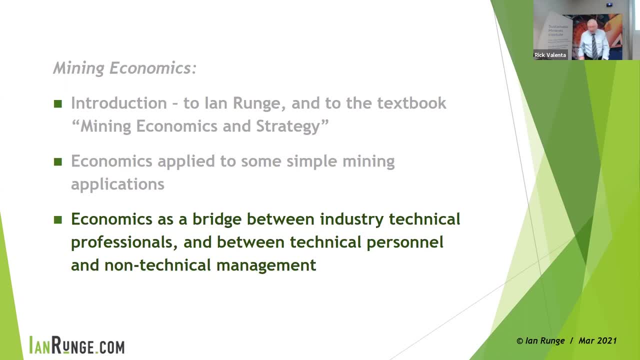 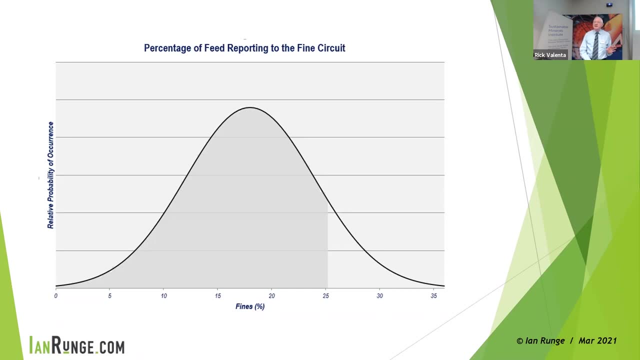 But this is a problem that occurs in many industries, but none more acutely in mining. It has to do with uncertainty, Some uncertainties you just have to deal with. Some uncertainties can be resolved by expenditure on more drilling, sampling, pilot planning. 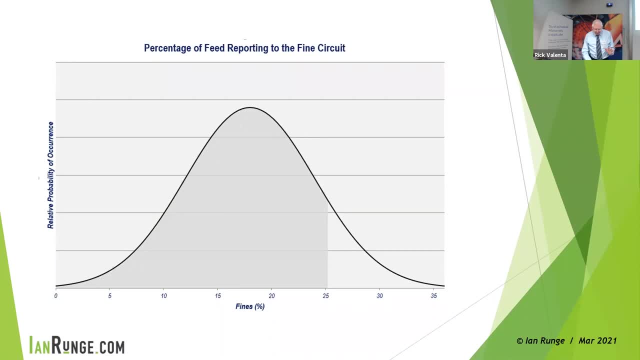 sampling, pilot plan testing, And some uncertainties can't be resolved regardless, like the future price of the commodity you're selling Now. take, for example: you're charged with designing a processing plant, particularly the fines processing And from preliminary studies. 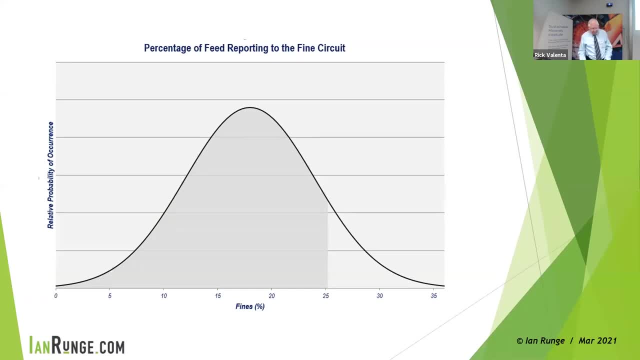 where we learned that our expected 18% of our feed is going to report to the fines. Well, we clearly don't design our fine circuit just to handle 18% of our feed rate. But what capacity do you design for? Do you design for covering 75% or 90%? 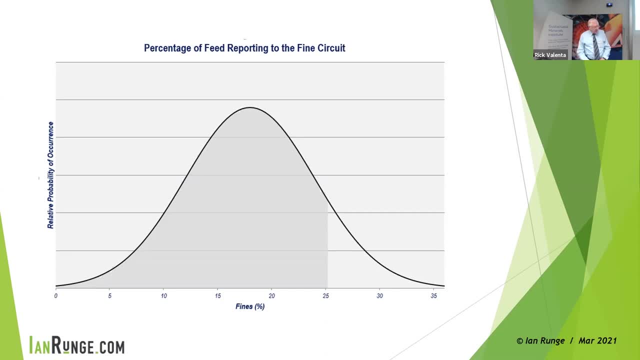 In this example I've drawn the suggested rate at the 90th percentile there, But you can use economics to work that out. If you are- first of all- let's assume we are- totally confident about that distribution, Then the rate to design the fine circuit at 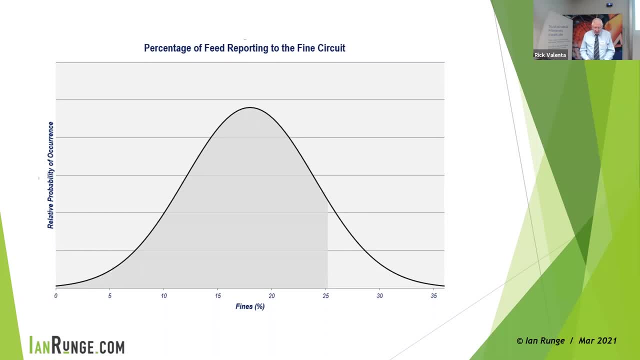 is actually quite simple, conceptually at least. You'd look at the marginal cost. Here's a whole economic mouthful, so get ready to digest. You would look at the marginal cost of processing each increment, based on the extra cost of the extra installed capacity. 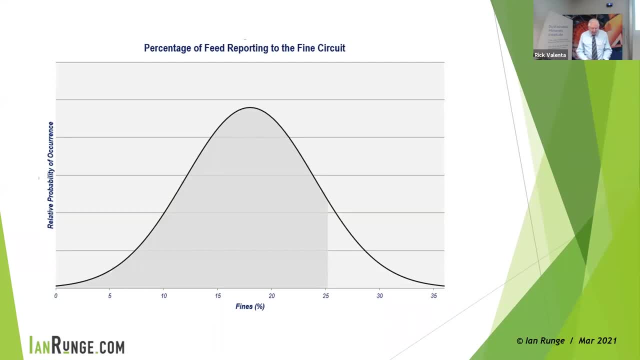 And consider the marginal return from the additional tons you get And you would design at the rate where the marginal return equated to the marginal cost. That's pretty simple, a big mouthful. I said simple and I meant conceptually simple from an economic perspective. 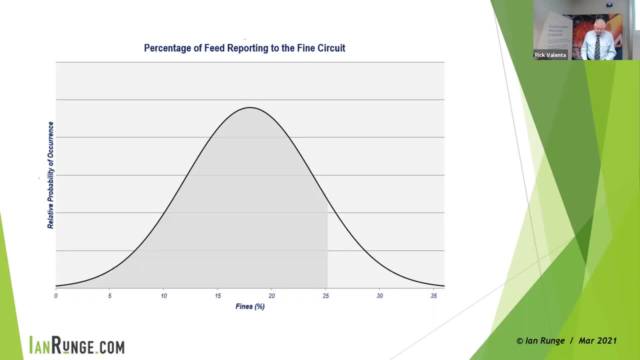 The calculations would probably be very complex And your design obviously can incorporate whatever you want in it: feed, stockpiles or whatever you like, But this is assuming you know the characteristics of the distribution. like owning a casino, There is variability but you deal with it. 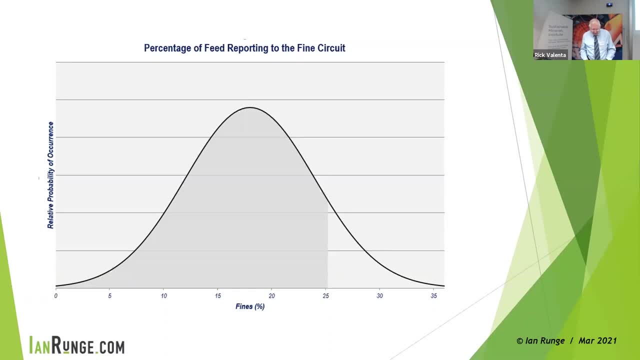 The economics field actually has some quite good tools for dealing with this kind of a problem, where the uncertainty can be expressed in some probabilistic way. But in mining we're seldom dealing with variability whose characteristics are known. We're dealing with nature's ore bodies. 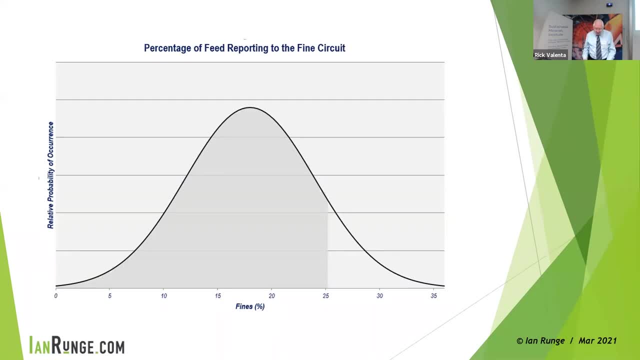 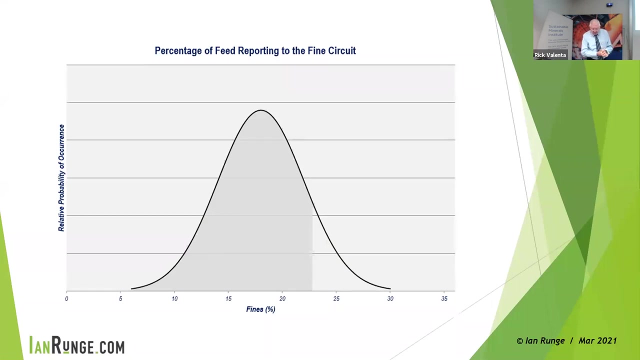 and if we spent more money on drilling, sampling, pilot plant testing, we might be able to reduce our expected variability. But now, with less expected variability, we can potentially achieve our 90% design capacity with a lower throughput or lower design capacity. 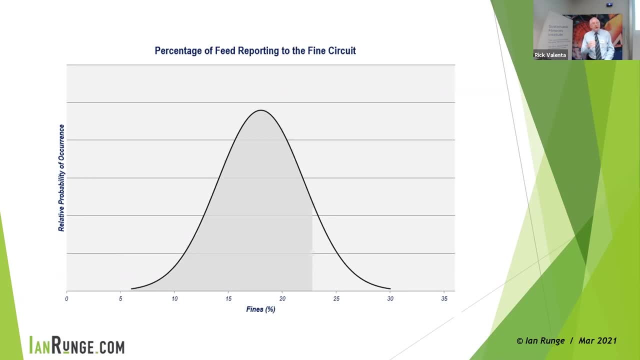 The savings in plant design might be significant, but how do you trade off the benefit or savings in the plant design against the additional cost of drilling, testing and sampling? Because you spend more money doing more drilling and testing and sampling, the distribution may not change. 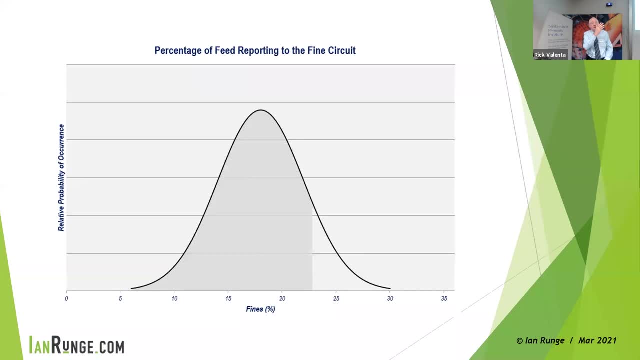 or the median, probably won't change. It might even get worse. It only changes your confidence in the shape of the distribution. So this is one of the big problems we have in mining economics. We can spend money to reduce uncertainty, but a mine plan prepared on the basis of less uncertainty 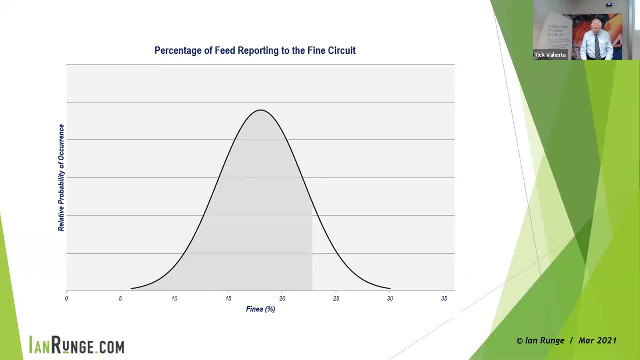 isn't necessarily any better From an NPV perspective. it probably could even be worse by the amount of money we've just spent on the extra sampling and drilling and testing. And I don't know of any mining company that uses different discount rates based on any quantitative measure. 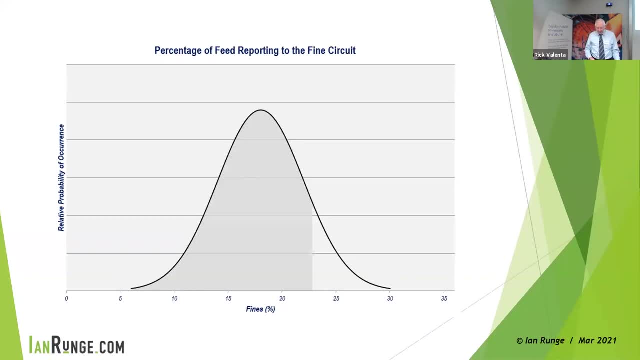 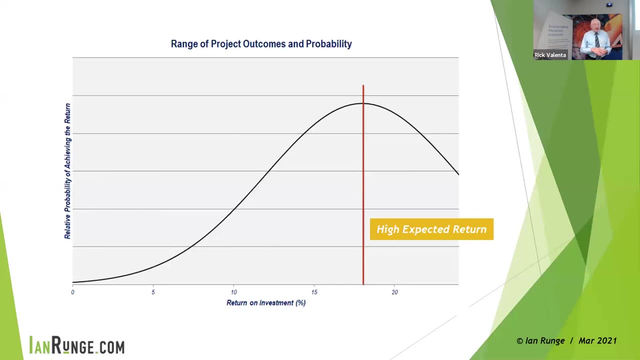 of uncertainty. You think of the process of discovering a potential mine and gradually proving it up. For example, a mining company might own some promising but early-stage exploration areas in some mineral-rich province. You could conceptually portray the value or return on investment like this: a potentially high return. 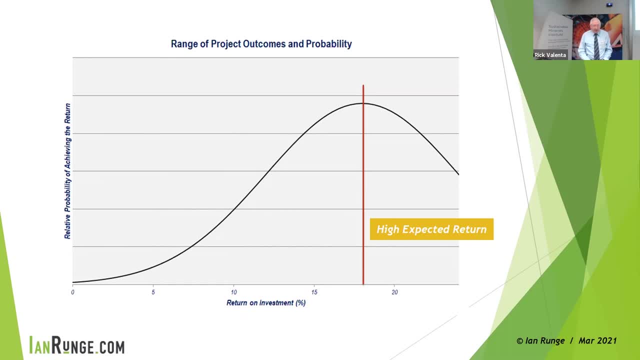 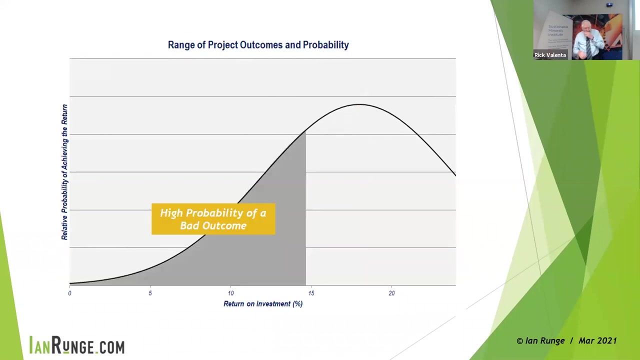 but potentially lots of uncertainty. Note that the project fails not when the return on capital investment is less than zero. It fails when the return on capital is less than the cost of capital In projects like this one, at this stage of our knowledge, 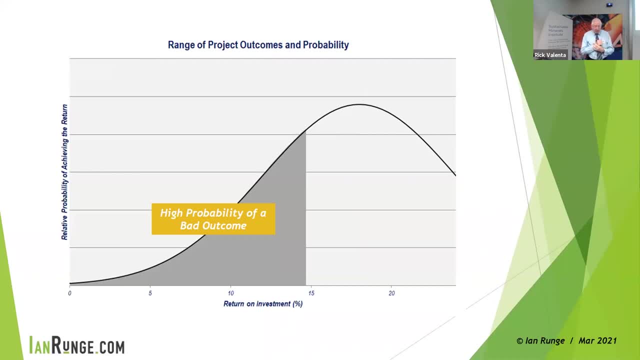 if we wanted to start it, the cost of capital will be very high. The process that ultimately leads to commitment is one of successive rounds of evaluation. Maybe there's too much risk- the shaded area- for this project at this stage, but we can spend a small amount of money. 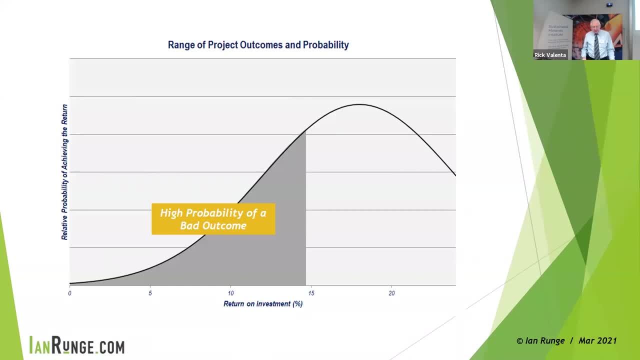 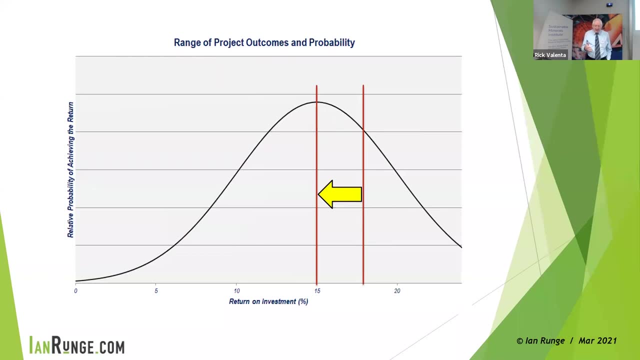 on exploration, for example, to reduce the uncertainty. Each successive round of evaluation costs more and more money- An ex ante, at least, before we go into it. it's only going to reduce the expected return on investment by the cost, by at least the cost of doing that work. 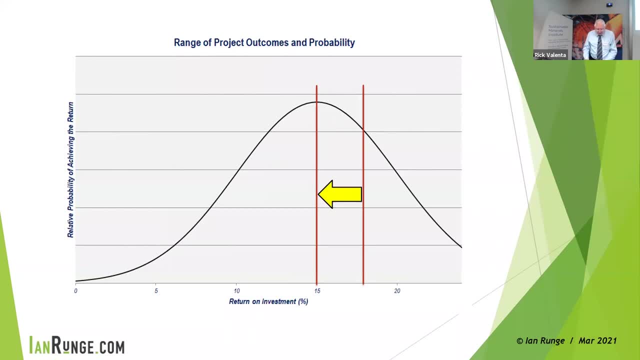 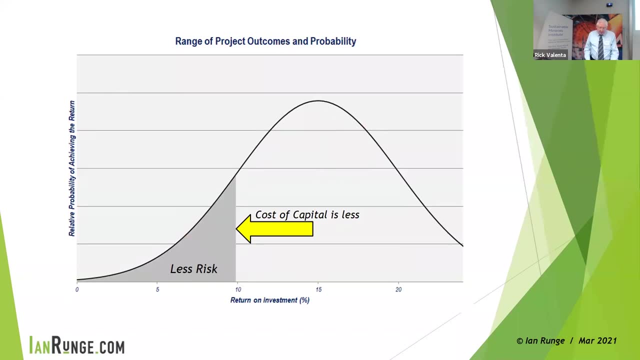 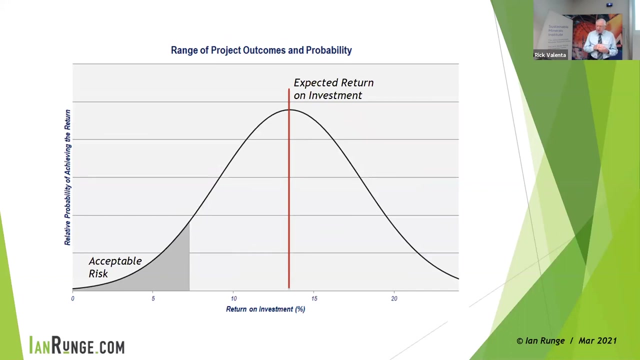 But as the project gets better understood, the cost of capital will also go down Until finally, hopefully, you'll have an acceptably low proportion of outcomes in the shaded area, while still having an expected return that competes favourably with anything else you might invest in. 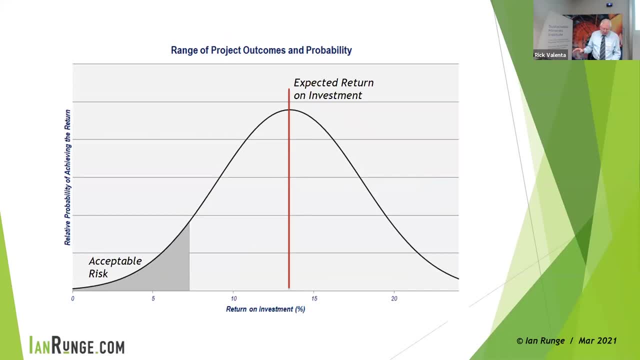 In this model and during this process, the focus is almost wholly on that shaded area. Well, I guess if you didn't have an expected return early on that was too low, well then, you're not going to get much of a budget to do more work. 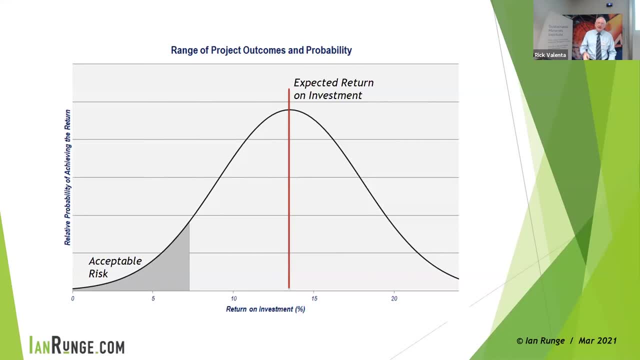 But, assuming you've got some expectation of a good return, all of the focus, all of our focus as technical people is on that shaded area And that's the probability of an outcome whose return on capital is less than the cost of capital. 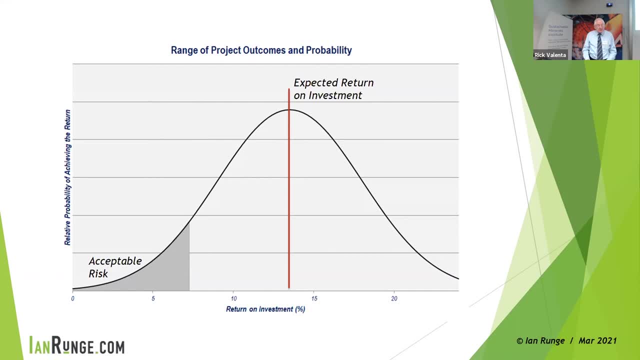 And I call this the uncertainty criteria. Any focus on expected return only happens after the uncertainty criteria is satisfied. Now the boards of exploration companies are totally familiar with this process. They make judgement calls every day about whether it makes sense to spend some more money on exploration versus the probabilities. 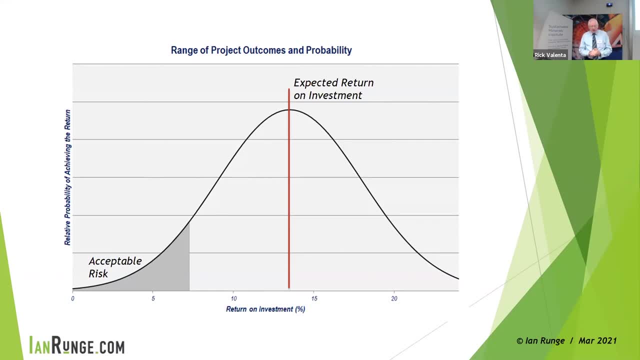 of either finding a better return Or refining the knowledge that they know about some existing ore body. The boards of mining companies are quite different. In my experience they know bugger- all about risk actually- But in my experience they implicitly assume when major projects. 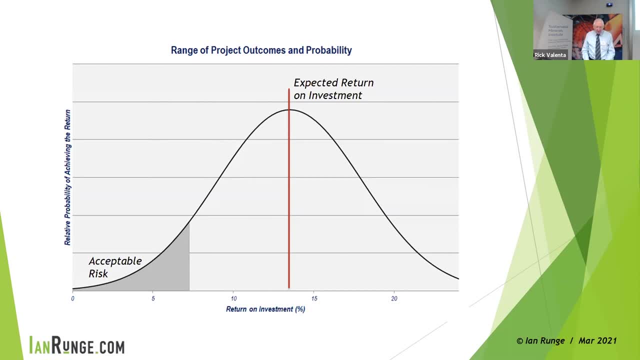 are presented to them that technical people have already done their work and the probability of the project ending up in that grey area is already acceptably low, at least from a technical perspective. If it's not, the project comes with some sort of audit review. 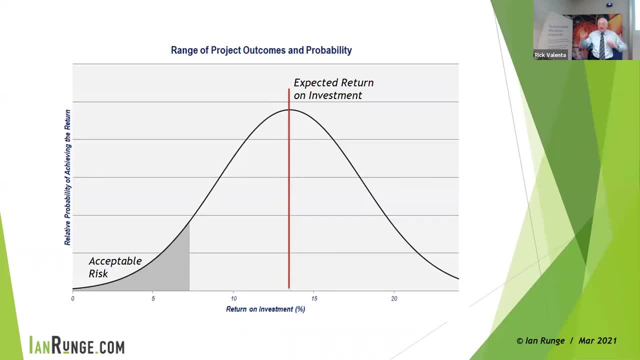 by some outsiders so that the board doesn't actually think about that. They've got other things to think about. Mining projects still fail, of course, some of them quite spectacularly. In the last two decades there have been many case studies to draw from. 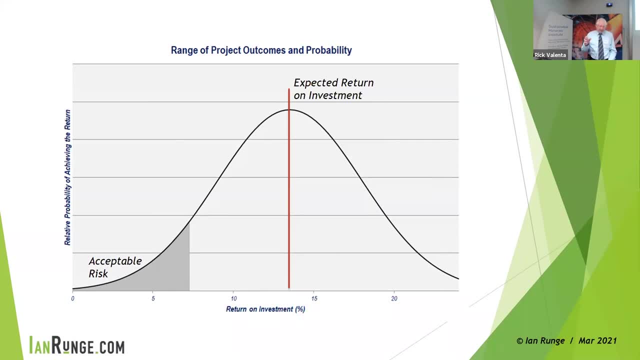 It's a particular interest of mine But, as I said, that's not a high note to leave the talk on. So I'll leave this discussion, that discussion, for another day, if you invite me back, And I'll stop there and invite some questions. 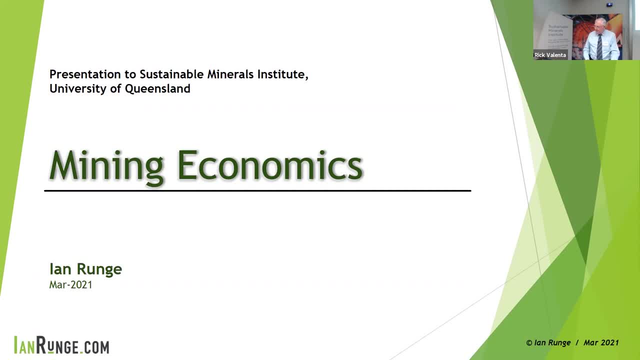 Okay, Neville's given me the task of managing the questions, So we have two different potential sources of questions. We have an audience here And I'll just please ask anyone in the audience. if you have a question, put your hand up and we'll bring the microphone to you. 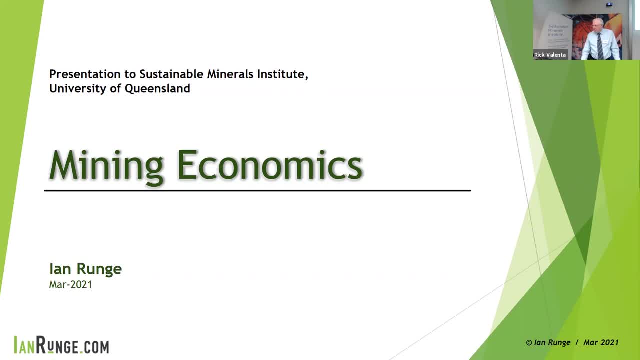 And meanwhile we don't currently have questions in the Q&A. but there was one point in the chat while we're And this came early in the talk, so it may have been addressed, but I'm too stupid to realize whether it has or not. 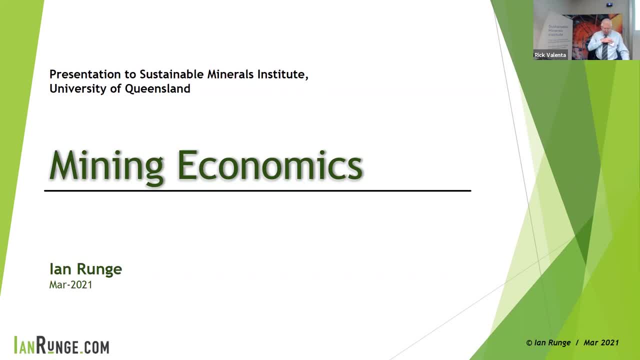 Early on one person said. one person made the comment that maximum yield doesn't equal maximum revenue. So while you're, If you want to address that question or that comment, then I'll leave it to you. In the meantime, if anyone has a question here, 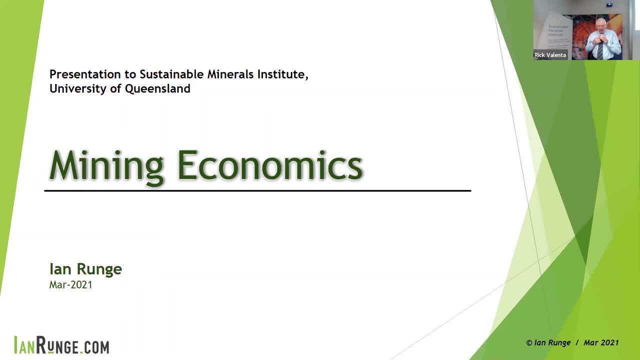 I'll bring you the microphone. Yeah well, I think that's totally correct. I mean, it's probably pretty close in a lot of cases, but you can maximize your yield maybe by reducing your grade quality or something like that. Sure, 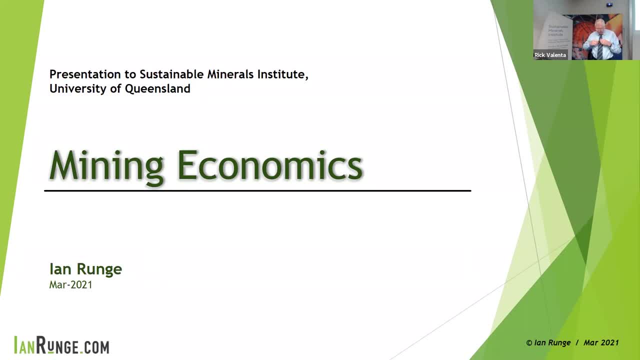 Brett Garland from the Mining Industry Safety and Health Center. Unfortunately, some of those case studies you'll mention at your next talk are more or not a couple of my projects whilst I was operating mines. But the question is: you've covered the mining economic side of it today? 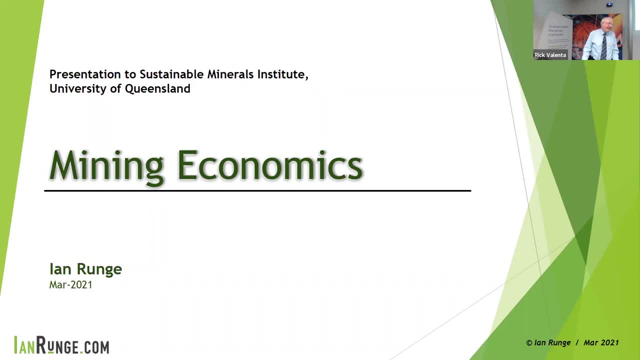 and economists, like mining engineers, are often pretty maligned, but economists usually end up in politics And therefore when you're looking at the life of a mine and the policy changes and the legal changes over the life of that mine, the economic uncertainty that they bring to a project, 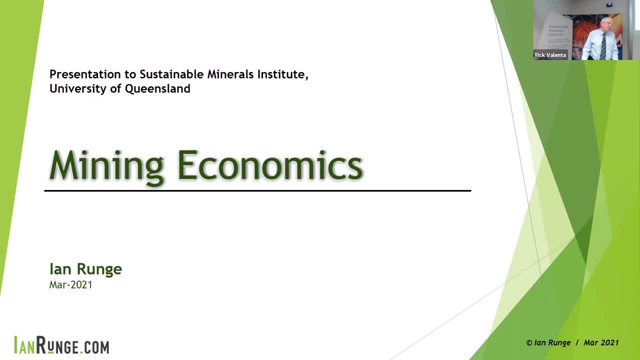 how do you bring those into your modeling and try to keep in that unshaded area? Ah, that's a good question And I think it's sort of It's the same kind of question. if you know, we expect that the price of copper 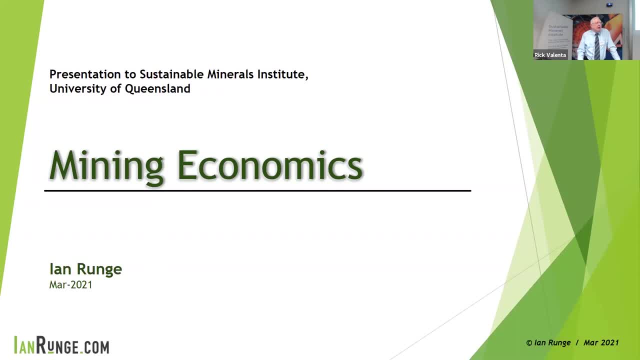 to be X now and it turns out to be lower than that. what do we do? And I think, Oh, actually, I think you can predict some prices better than we do- Not real well, but, And I think you can almost predict some of those policy changes as well. 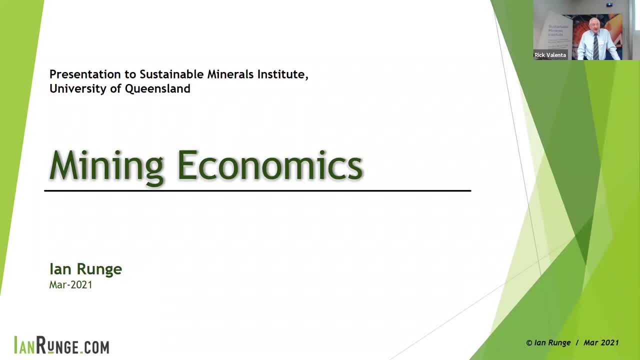 or at least you can be alert to a scenario like that. And one answer to that is: when you're planning a mine, or When I say mine I mean the plant or anything else about it- One of the things we've got to learn is the mines that had scope to change. 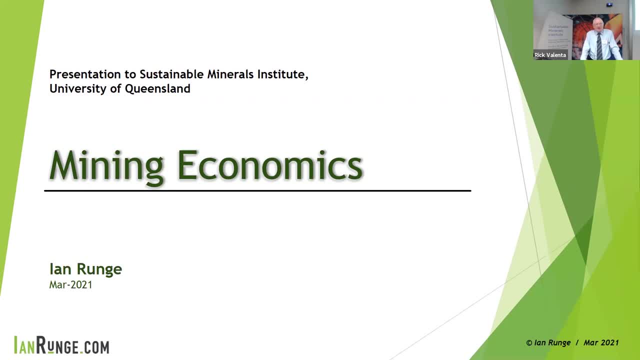 have handled that much better than the ones that haven't. So I say to people: okay, we're planning this mine. Are we shaving the last dollar And is the One of the prices we're paying is our inability to change, And I think 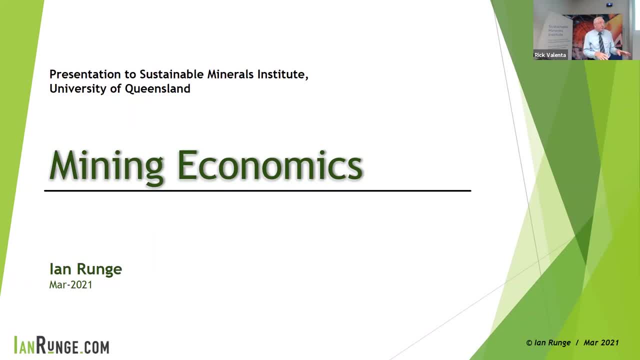 And that might be a choice of what we're doing in the mine. It might be a characteristic of the deposit. For example, there was a nickel mine in West Australia And I'd done some work on it And I'd said to the company: this is not a go. 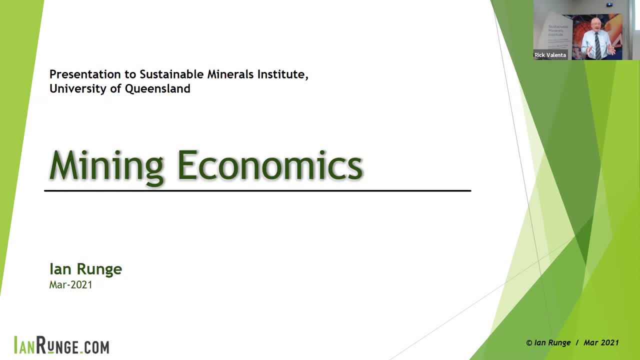 because there's just not enough reserves there. So if something happens, there's nowhere to go. For this mine to work, everything has to fall into place, And it's a long story. but the company started and it failed And they wrote off a couple of billion dollars. 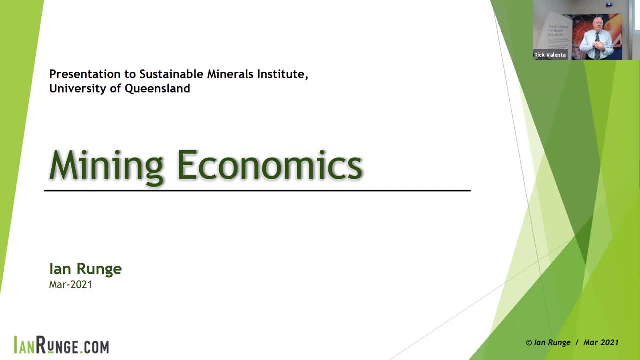 And whilst they didn't blame that for the issue, they blamed the lower nickel price. But in fact, a mine developed on a different kind of deposit that allowed more scope to change wouldn't have been hit with what we got. And you know, you can see it. 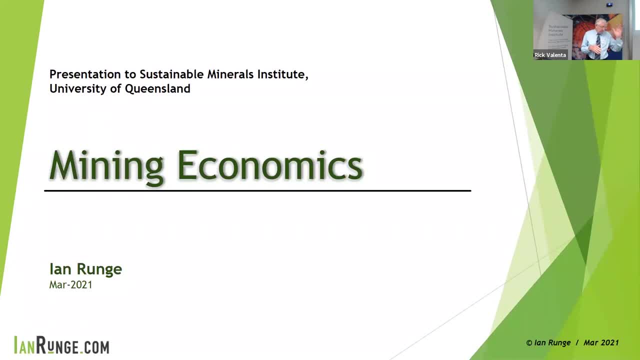 There's a high price of something, The price falls down, The company gets into cost-cutting mode. They fire everybody there who's not involved in production, including the planning people, And they reduce their inventories in the pit so that they haven't got enough scope to blend that type of ore. 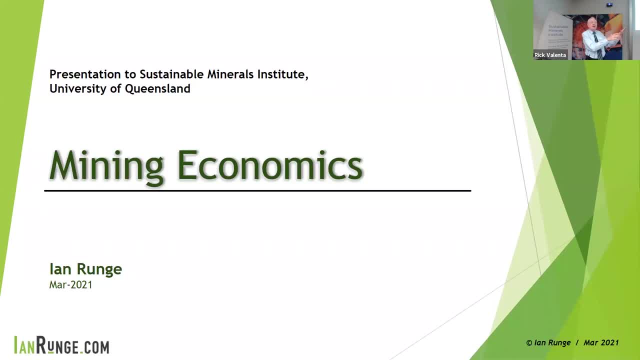 with this kind of ore, And then next minute the market requires some other change and they don't have the scope to do it. And not only that, they don't even have the personnel needed to replan the mine, to know how to do it. 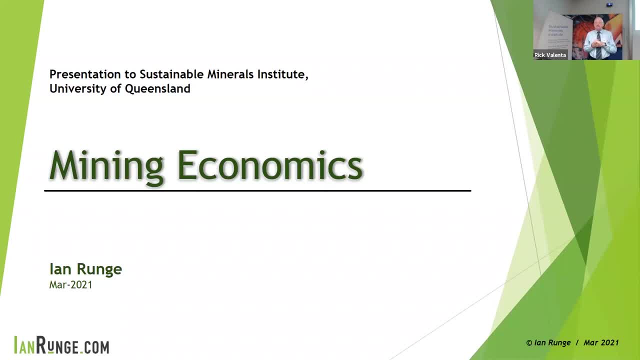 And the next minute they're caught out and, you know, something bad happens. So I think one answer to that question is: we don't in our planning, we don't have a good mechanism to value mines that have got scope to change ahead of mines that have less scope to do it. 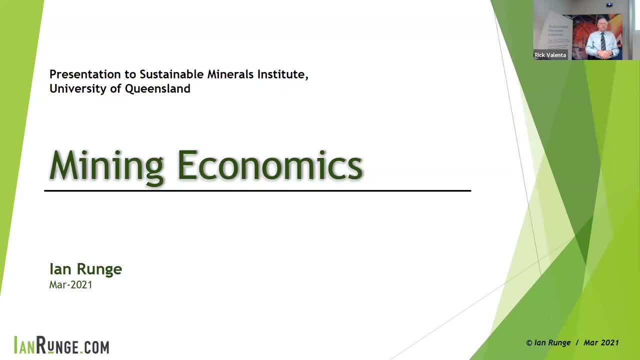 We have to have less scope to change. Okay, We've got a flood of questions online, So I'll do another. I'll do an online question, then move to another one in the audience. So the first one that came in online was: we'd love to hear your comments. 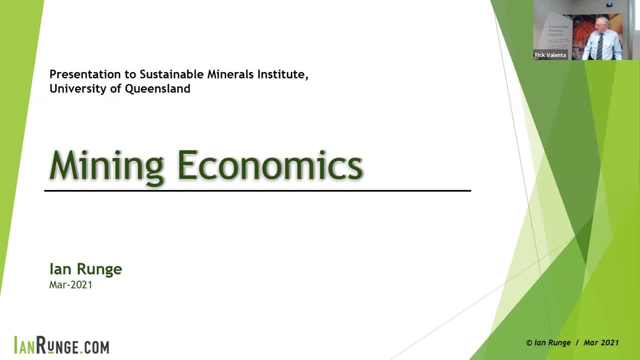 on building planning for mine closure and mine rehab into marginal costs? Ah yes, That's a well, that's a challenging question. Thank you for that question. I'll just stall another minute while I think of a good answer. I think every plan that we do nowadays we take into account mine closure costs. 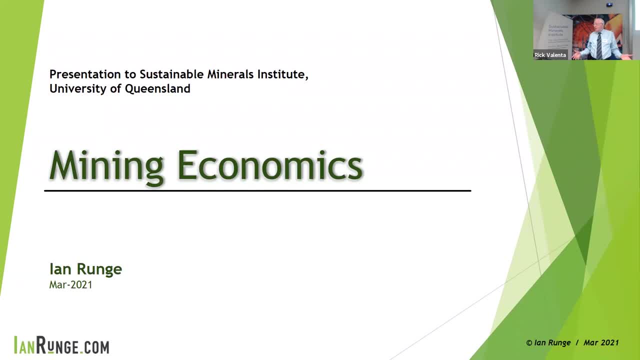 But if you're doing a discounted cash flow and the mine's got reserves for 48 years, the present value of a lot of that is nothing, or the present cost of that, And a lot of people are uneasy about that because it's essentially 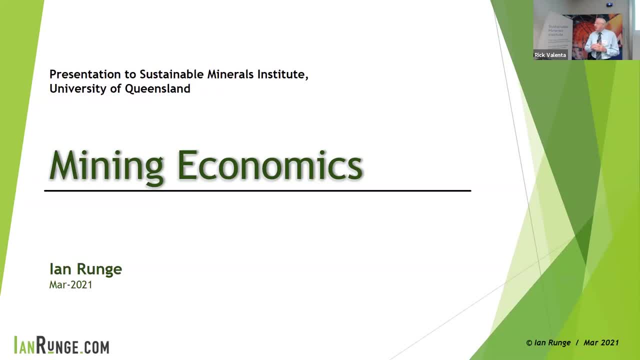 if that's the way you're thinking of it, it doesn't change what you're doing now. Well, in one sense there's some correctness in that, actually, but it doesn't happen until then You've got when the mine is operating. you can do a lot of things in the interim. 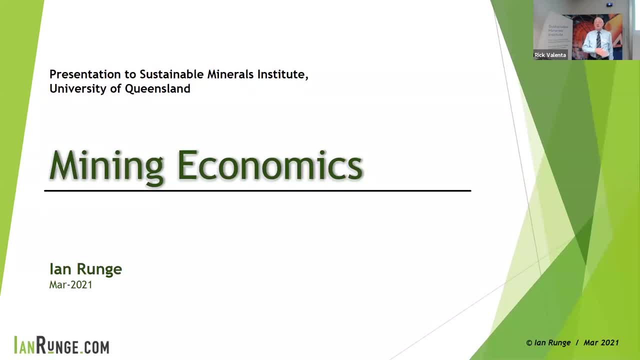 And particularly if you've got time to, if you know it's going to close in 10 years, then you've got a lot of work Because you're moving a lot of material around for those last 10 years. you can do a lot to it. 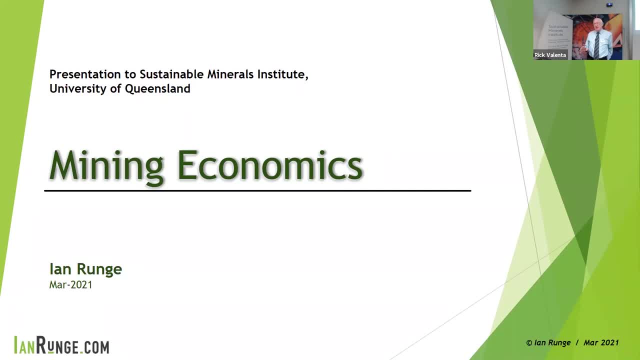 So my experience is that those costs are not you take into account. they're not that high so long as you know about them in advance and plan around it. It's when someone changes the rule on you and you have to do it now. 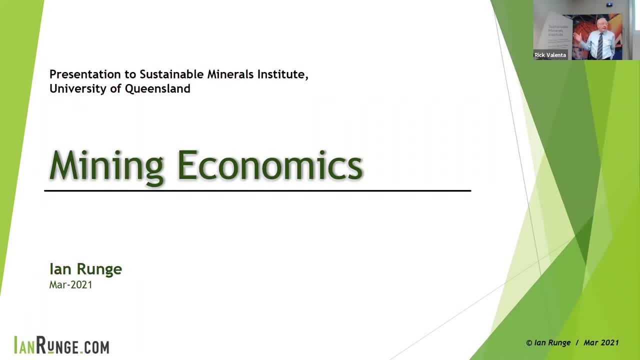 then all of a sudden you find you're in a $500 million write-down because of some valuation change. Incidentally, this is a another thing about that we don't look at with a lot of mine plans is we plan mines as if it's going to keep ticking over. 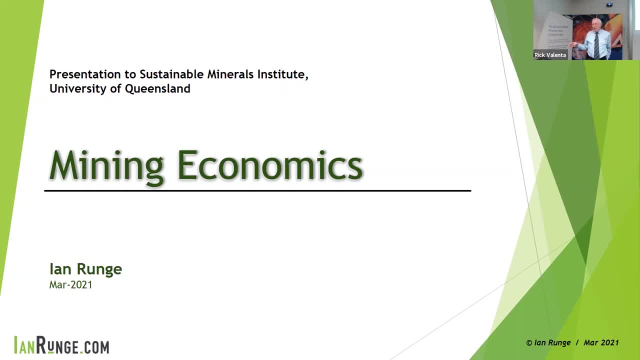 And we don't put a lot of cognizance on the issue of if it stops ticking over. So, for example, if the mine is keeping on going well, then it's easy to do that rehab because you've got truckloads of material every day to fill it in. 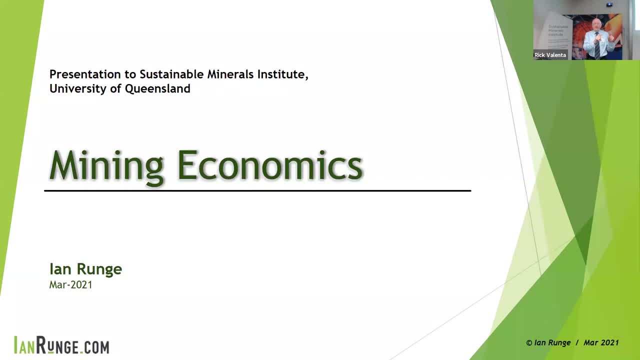 If the mine doesn't tick over, then the cost of doing that rehab in a non-operating mine might be millions. I was involved in a mine in central Queensland where that happened. The accountants had made provision for about $1 million of rehab costs. 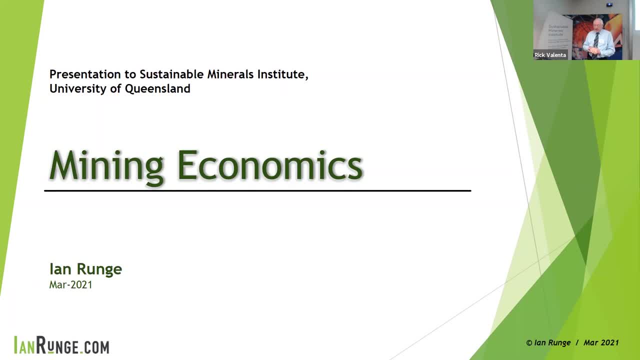 under the assumption that the mine was going to keep going And then when it closed down, bought by a new owner, the old owner had that provision on their books so they guaranteed that rehab. But then they discovered that that new owner wasn't going to mine. 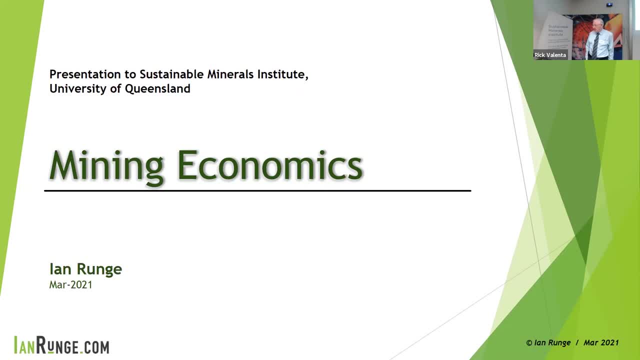 that part of the mine anymore and the rehab cost was like seven times. So yes, Let me also tell you. you know, when I worked in the UK, this mining company, we actually had a final void and it was only a short-term contract, four or five years. 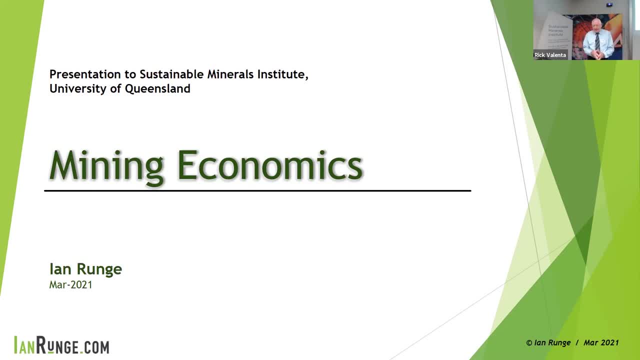 so we knew we'd have a final void. But keep in mind that that final void- the company made more money out of that final void than they did in the mining because it was an established area and there's nowhere else in that established area for disposal of garbage and crap. 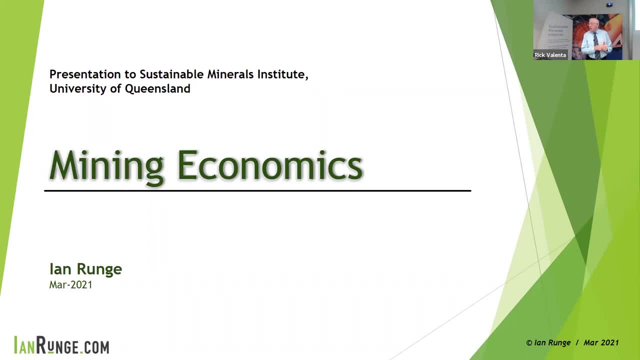 And so it was actually a very profitable thing having a final void, And I think if you're in established areas, some of those things that we think of as liabilities can actually be assets. I hope that answers the question And Marcin Zemski from JKMRC. 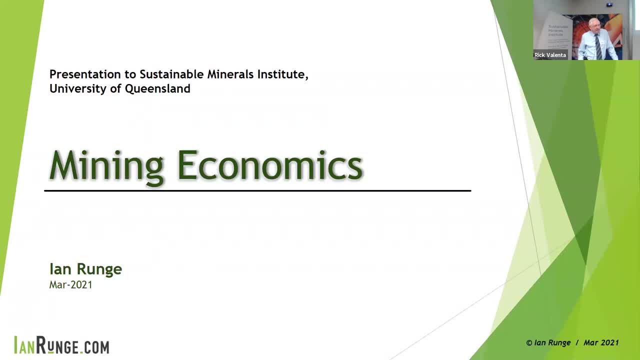 And I think this is partly linked to that previous question. What are your thoughts? You mentioned economics a few times and the power of it, and that we should be careful and apply it well. What are your thoughts on the application and use of NPV? 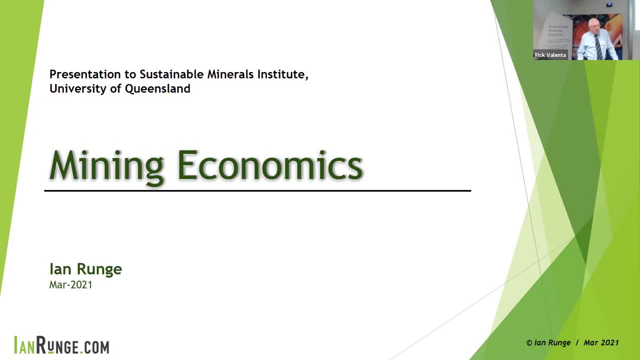 as a measure for mining decisions. Is it valid? Is it something that is the only way to go, Or is it something that we should relook at, especially given the fact that these mines often go for 10,, 20,, 30,, 40 years? 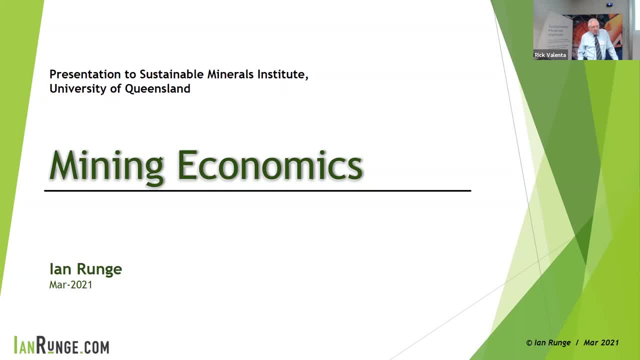 and NPV only actually gives you an insight into the next five to 10 years. Okay, that's a good question. Should we use NPV or there are some other measures? and to what extent does the NPV not really properly consider some other issues because of the too far in the future discounted? 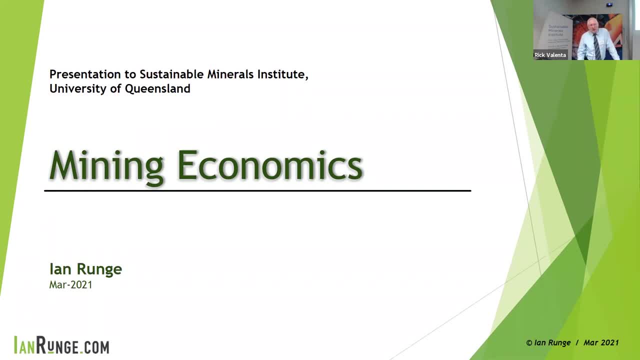 market. First of all, I won't get into arguments of NPV or IRR or those. Frankly, if you can give a project the go ahead or not go ahead on the basis of one difference or the other, then don't do it. 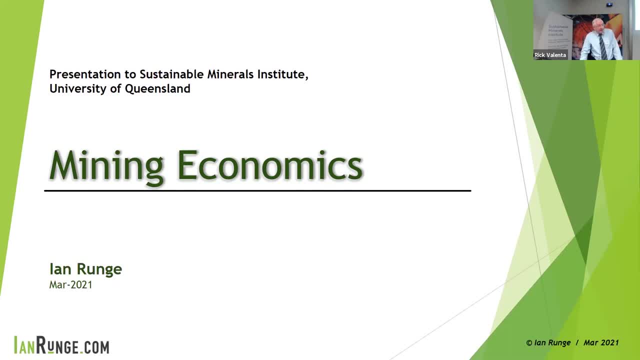 Mining projects need to be pretty clearly a goer, Otherwise don't do them. That's what my experience is. The companies I've been involved with that have tried to refine those numbers and argue about NPV or internal rate of return. they've lost the plot. 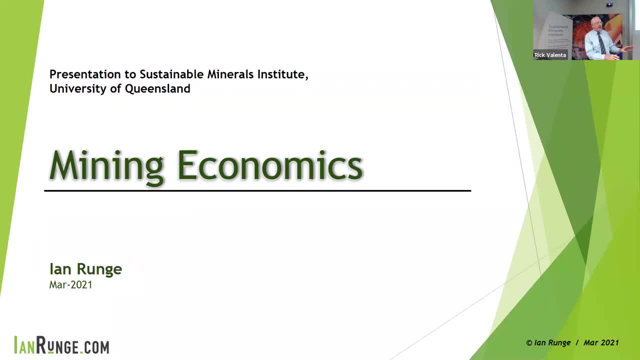 It has to be a good thing, make sense rather than any academic argument on IRR or NPV. But you've got a valid point in the sense that some of these things are worth looking at more than we look at them Like: what discount rate do we use? 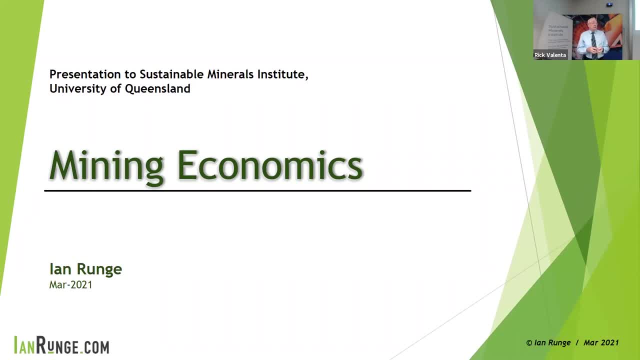 Well, you know, if you're up in central Queensland and want to start a business in coal mining and you've got a huge history of mining and the technology and it's one mine and your company's already got six other mines, then that's a whole different thing than if you want to start up. 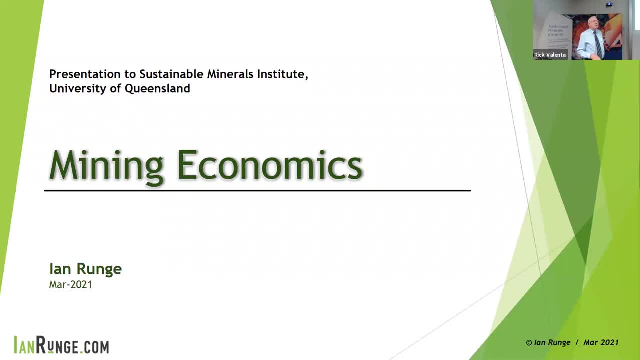 a graphite, mine in Gaborone. So we have no good mechanism to say, well, the discount rate here should be 8% and over there should be 15.. Where do those numbers come from? I don't know anyone who's got any kind. 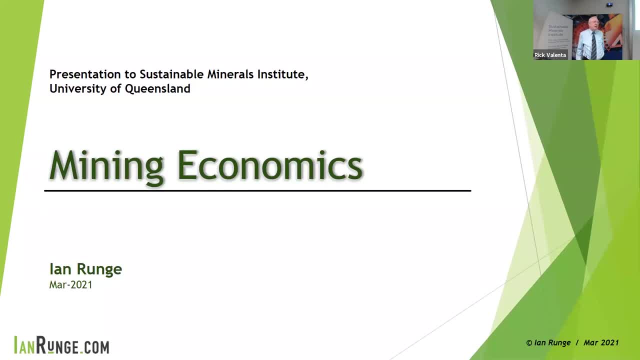 of mechanism to quantitatively do that Also, I think there's an issue too is that things that happen sooner have less risk than things that happen further down the track. But we use the same discount rate. We shouldn't. You know, if you want a loan, if you've got to invest in government bonds. 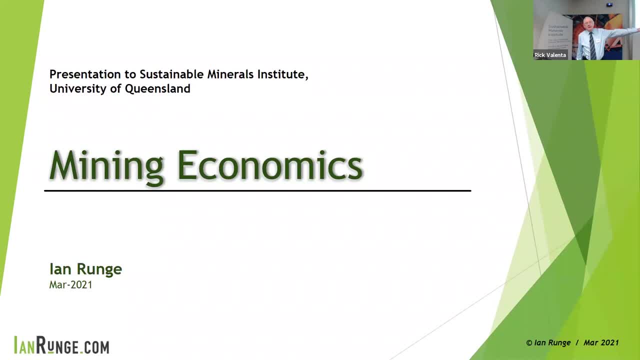 and it's a five-year rate or a 30-year bond. the rate on the 30-year bond is higher than the five-year bond. Therefore, the marginal rate of stuff further out is much higher than the rate of stuff further in. So stuff further out needs to have a higher discount rate than stuff closer in. 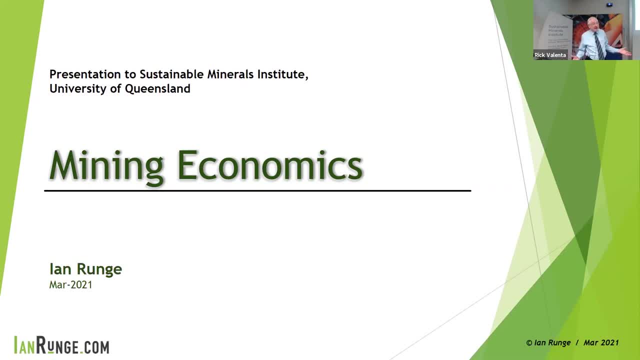 I don't know anyone that uses differential rates as a function of time out. Same with things like well depreciation allowances, which gives you tax benefits. I mean there's no risk in those. They should be discounted at a low rate. 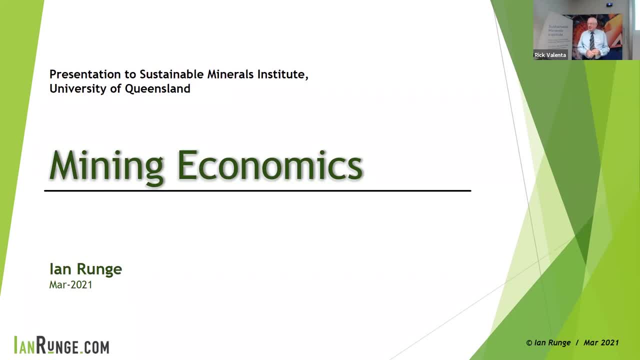 I don't know anyone that uses differential discount rates for different elements of the cash flow. frankly, Some have played around with it, but I don't know whether that answers your question. I will be looking in my new book some of the talk about investments based. 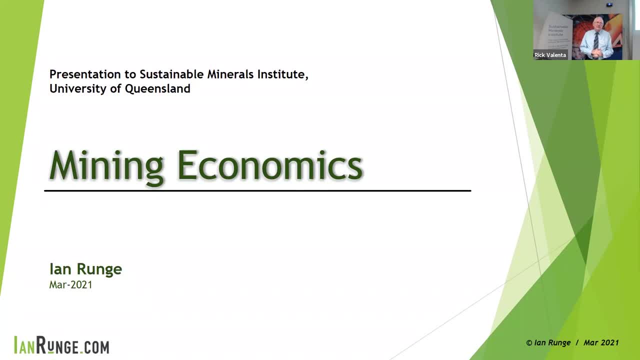 on different discount rates. Does that cover this? Yeah, So we've still got seven questions in the Q&A. I suspect we won't get to all of them, So I thought I'd jump straight ahead to one that's controversial but probably topical, and that is from an anonymous attendee. 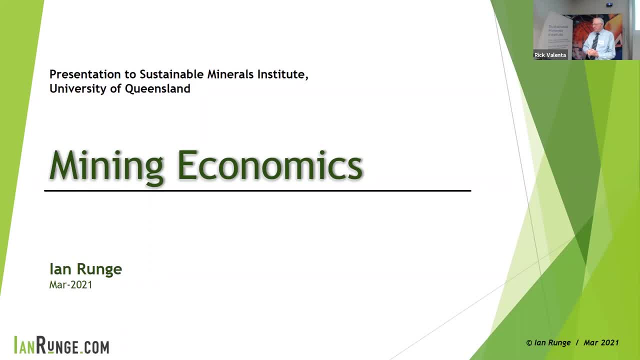 Ian, in your experience, what does the demise of the mining engineering profession mean to the industry? What is the demise of the mining industry, mining profession? That probably means that those are the ones who have still got the skills are going to get paid more. 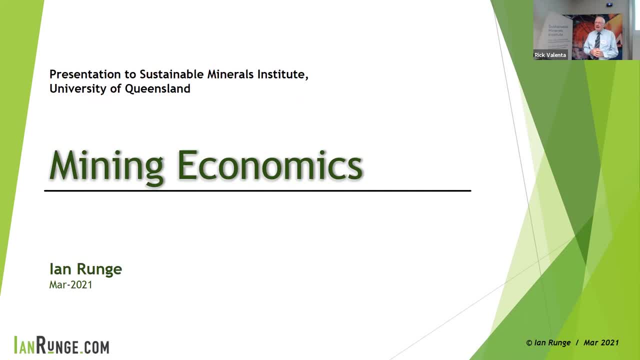 That's the way an economist would work, I would say. the bigger question there is that in times past, the managing directors and the bosses of mining companies were people who grew up in the mine. They had done their time at the coalface, And so when, as a manager, they're called upon something, 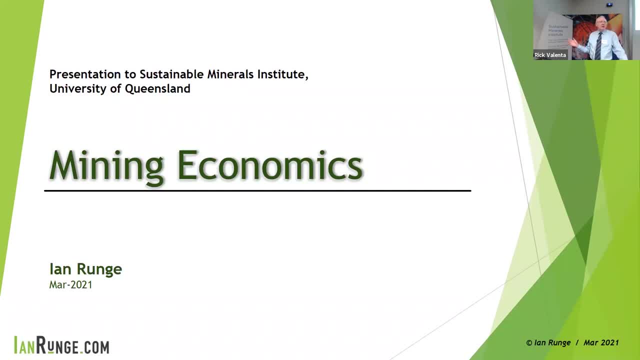 they had some of that gut feel. I think our management now in the big mining companies has almost none of that And I think a lot of what I consider to be ill-informed decisions are an outcome of that. They go to Harvard Business School or something. 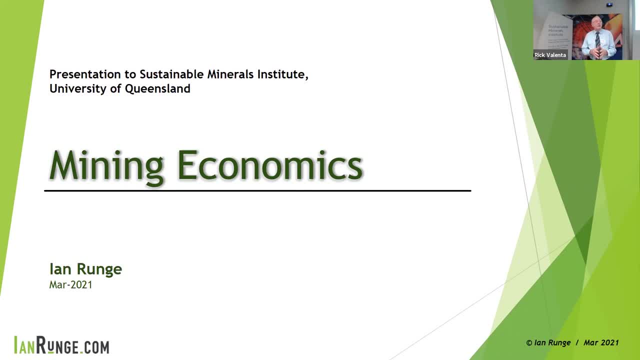 and they learn business practices that don't take sufficient cognisance of the kind of risks and uncertainties that are in the industry. that somebody who grew up in the industry did Now. I think it's fair enough. in the past we had senior people whose skill was production- running their companies. 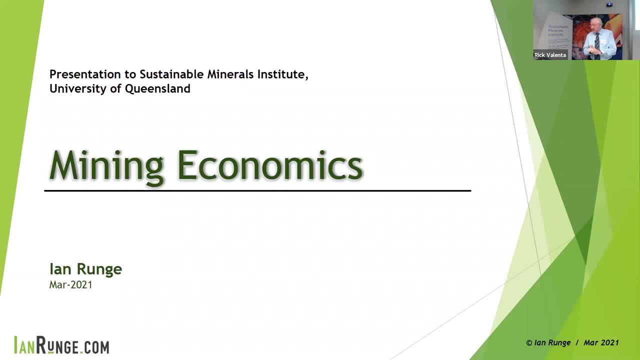 and often in not as business-like commercial way. But I think we've gone the other way And the biggest area where I think we've suffered is in the area of risk. If you grow up in the industry, you have a gut feel of what the risk is. 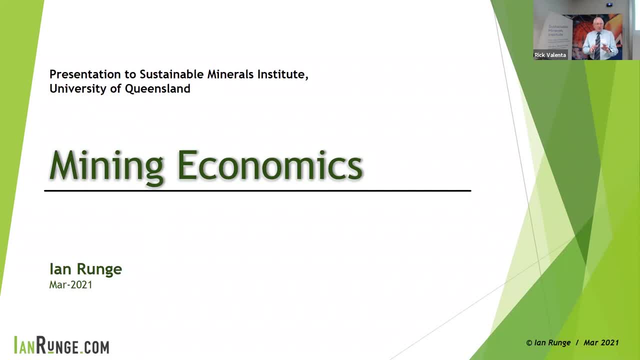 it would be great if we could quantify that better, And I'm hoping with my book and that's one of the things I'm doing. but at the end of the day, the buck stops at the very top, And I think one of my recommendations for people. 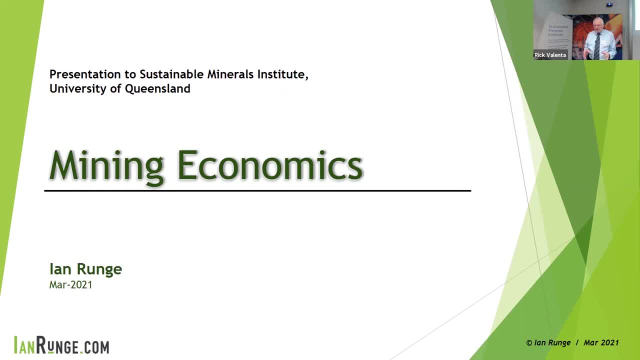 who are going through the mining skills is we need more mining people who've got that experience and get them, you know, restore some of that balance at the very top of our companies so that the people there are Of course. We've got some of that time spent at the coalface. 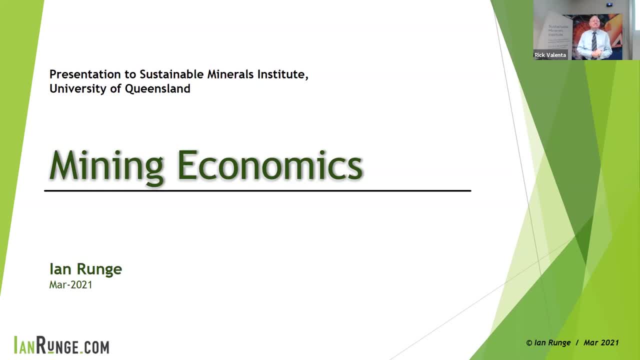 Thank you, Yuan, for a wonderful talk. My name is Vladimir. I'm from JKMRC. This place is, I mean, our small piece of jiggle. bigger picture is to improve the process, to improve efficiency. During the mining boom, there was a lot of talk about decline of productivity. 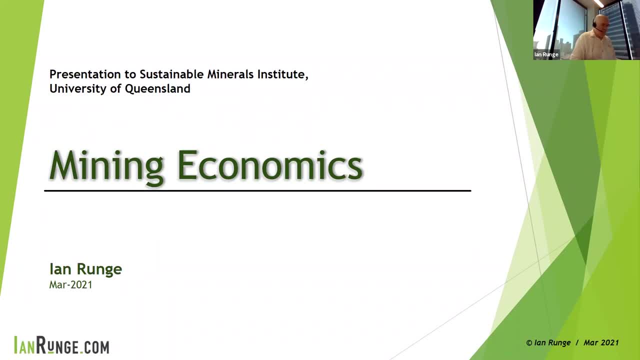 There were some people who were talking that we stopped mining smarter, or. my question is: we heard a lot about that. We heard a lot about the mining costs from you and processing costs. What are your thoughts whether that decline in productivity in the past? 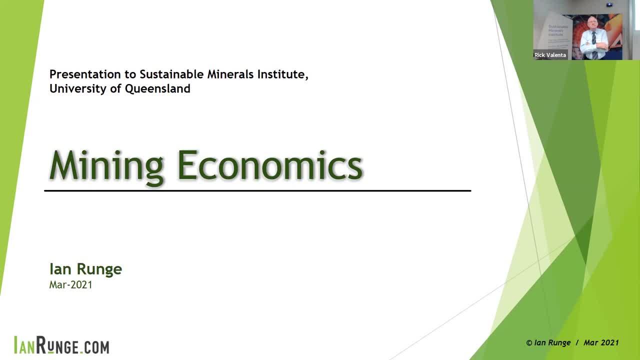 during the mining boom was due to inefficient processes or was it due to financial decision to increase the profits? Okay, So we're talking about efficiencies And in the boom there was less interest in that, And so you know, is there a real role for us? 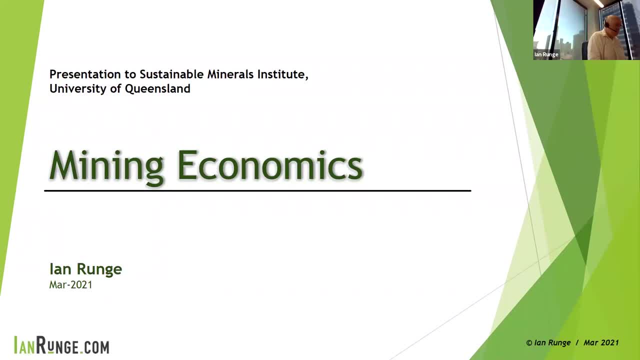 Yeah, if you're an iron ore miner and it's costing you $18 a tonne to put that tonne on a ship and you're selling it for $120, then it's pretty hard for us to come along and say, well, we can reduce that $18 to $17.50.. 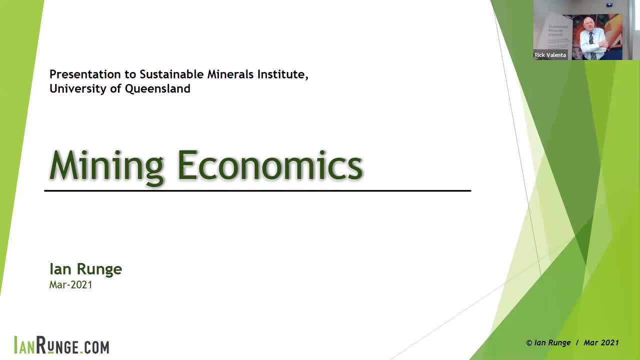 Buy better. You know a handling cost, isn't it? And so the focus then was only on tonnes. It didn't matter whether the $18 went to $20 or $30 a tonne if you're selling it for $100 a tonne. 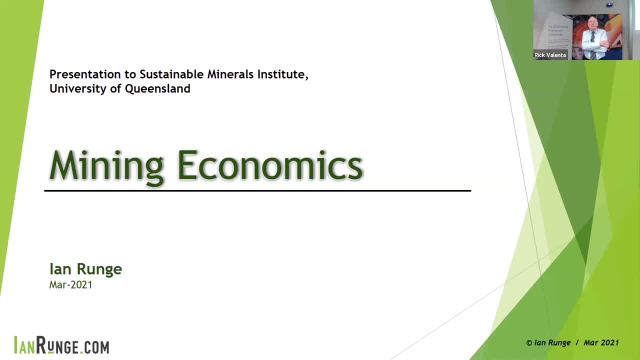 and you can just get some more tonnes out there, Then the bigger picture is this: I mean, this is the industry. It's always rooms and bus, and when it goes down they're not interested in efficiency, They're only interested in surviving. 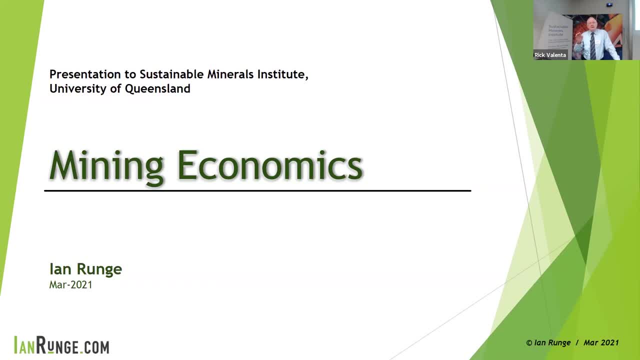 So if they're not going to focus on efficiency in boom times- and they're not going to focus, they're only interested in cost cutting in the down times, then that doesn't leave much of a window, does it? I think that's another artefact of our changing time, where you know. 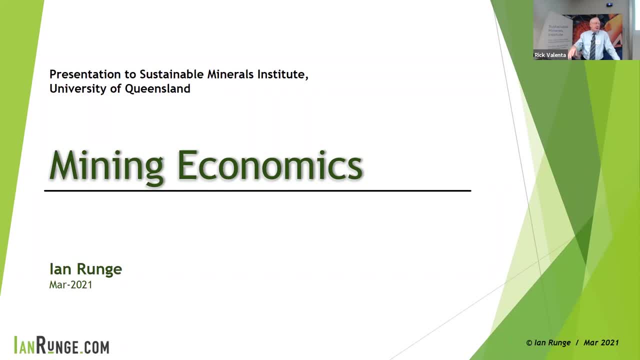 this centre was funded by Mount Isa mines and JK s era, when they recognised that there was some investment in long-term returns and the people approving that investment were the you know MD of those companies and they understood where it would pay back. 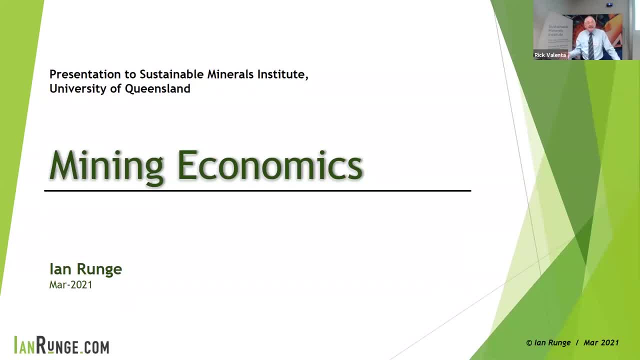 They could never do a DCF on their investment in the JK Centre. But some of these things are not going to happen. Some of these things are not, you know, able to be put into a DCF, any more than some exploration company can go out there and put some drilling. 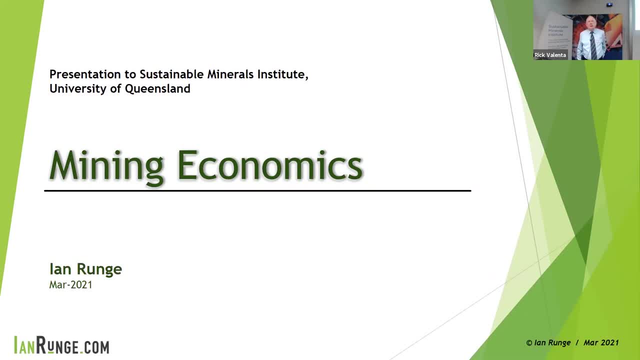 and have no clue whether they'll find something or not. I think one of the outcomes of this fact that our mining companies are run by professional managers without that mining technical background. it's hurt our industry, at least from a technical perspective. I don't know whether that answers your question. 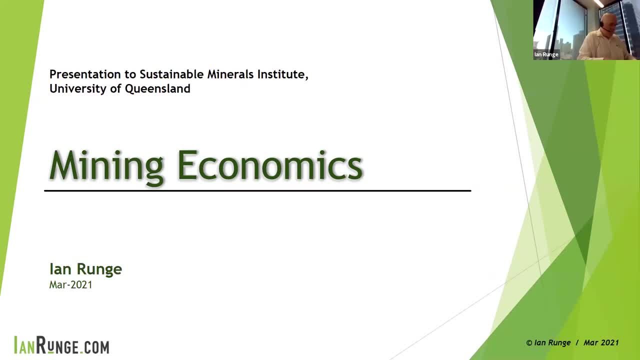 I think one of the hard things for us in this field of trying to improve technology or, in my case, better decisions, is that if the company uses poor technology or makes a bad decision, often you cannot tell that ever that happened, You can't tell. 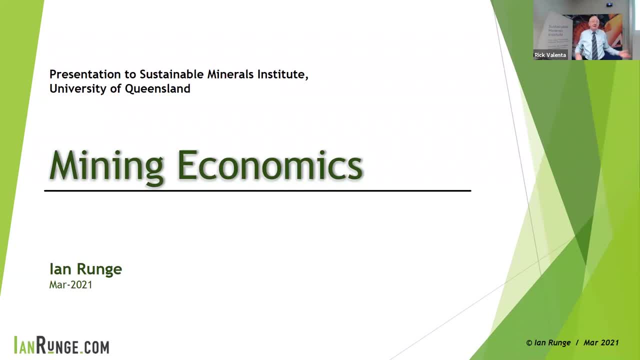 You can't tell that they could have made some better decision. And I've been involved in a whole bunch of mines in my life where I thought it's dumb starting that up And then, sure enough, something goes wrong. But they don't blame that issue. that I said was dumb in the first place. 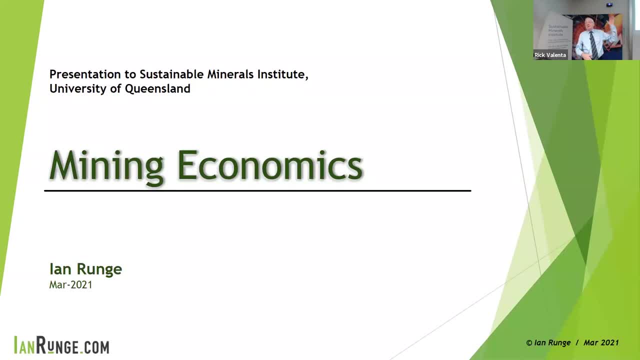 It's something else has happened. The price of the mineral has gone down or something else has happened, but fundamentally they made a mistake. We're just never, ever tying that mistake to some piece of technology. Maybe we've got to be marketing our skills better. 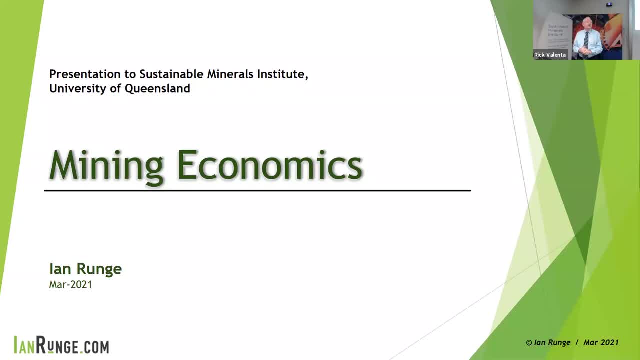 I don't have a long answer. That's a long answer. Sorry, that's a long answer. I don't have a better one, though, Yeah, Okay, So we've gone a little over time, but I think there's a lot. 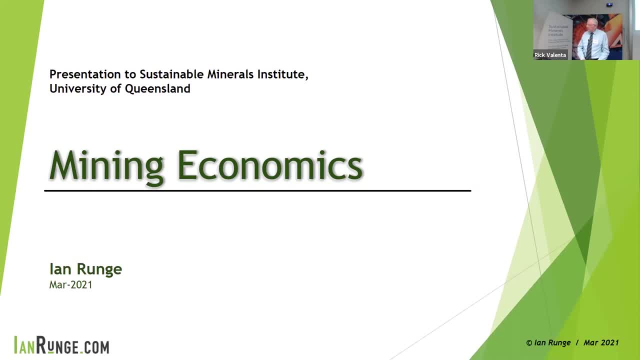 of good questions there And, as long as you're happy to keep going, we'll do one more from online and one more from the audience. I'm on double time now, So there are quite a few questions around the sort of risk and uncertainty. 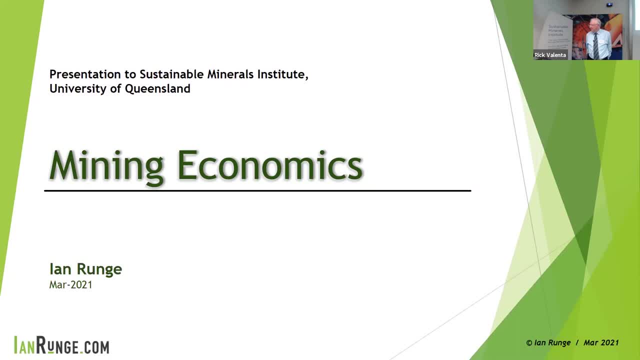 and future changes and that sort of thing. But there's one that I wanted to ask and that is in relation, again in relation to mine closure, or I think you could extend this to any event: really, what do you think would be the impact or how would you treat the? 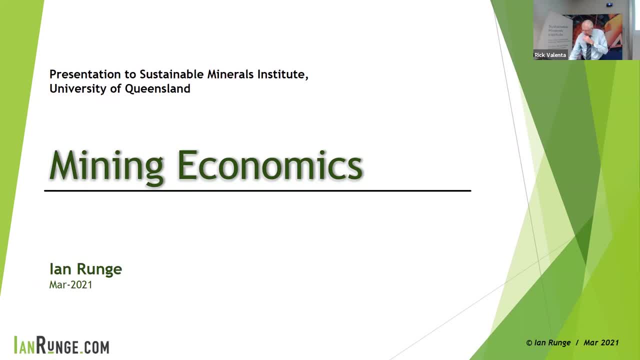 likelihood of a change of rules as an uncertainty In your economic decision making- And this is in relation to mine closure, but I guess unforeseen future events Could it sink a project's viability to these sort of future developments that are beyond the scope of your assessment of the project. 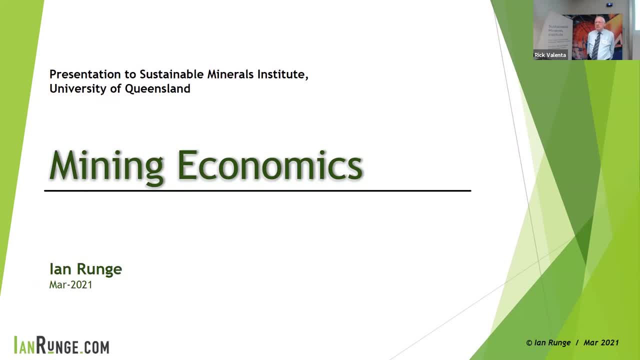 Yes, that's a good question. Is the uncertainty of a likely future change in regulatory environment or something sink a project? I think the Uncertainty sinks more projects than you know. if a regulatory environment said we're going to, you know. 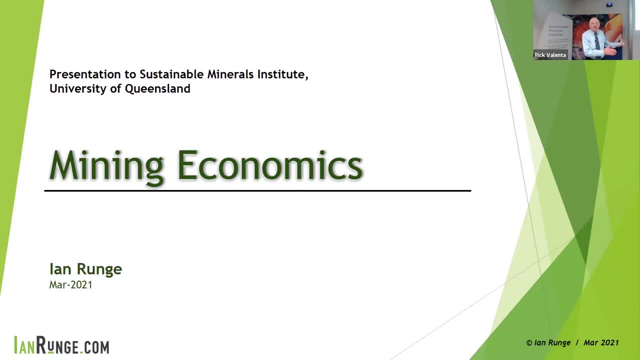 charge you X dollars per this, per that. if you do this, That wouldn't sink as many projects as the uncertainty of not knowing what they would do. You could use this example of travel in Australia with the COVID is: we'd like to go to Melbourne or something to see something. 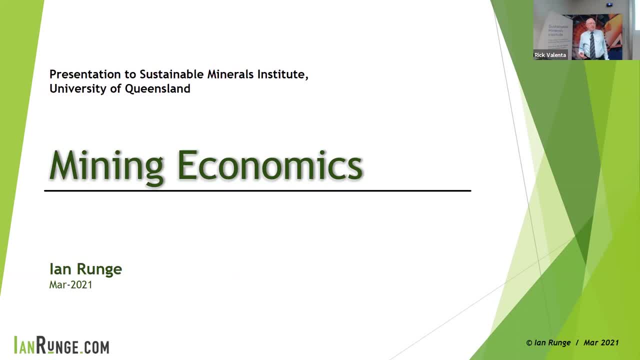 with some relatives, but if, on the risk of, like, closing the border on, you know, three hours' notice, we might have to do two weeks' quarantine, we're not going to go to Melbourne And it's not the regulation that's the problem. 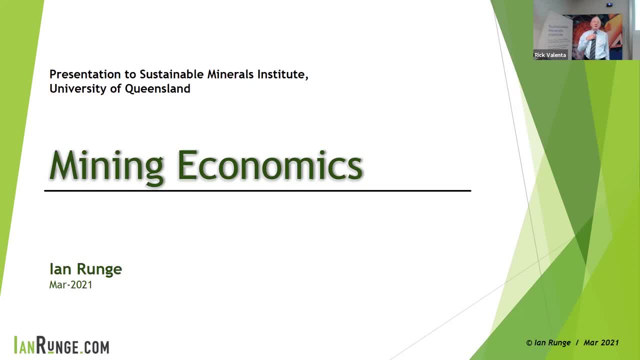 it's the uncertainty that stops us doing so many things, And I think that's absolutely the case. I think we start up a mine, we make a commitment. we can't you know if something goes wrong, And this is where mining is quite a lot different. 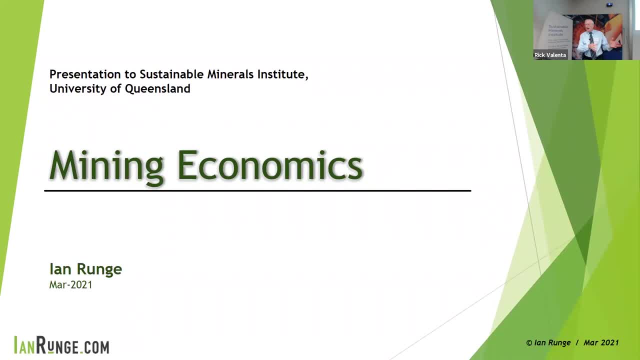 than most other industries. If you've got a car factory here and they change the rules on you, well you know you can sell the factory to make baked beans or something. your at-risk capital is a lot less. But in mining, once you've sunk that shaft, 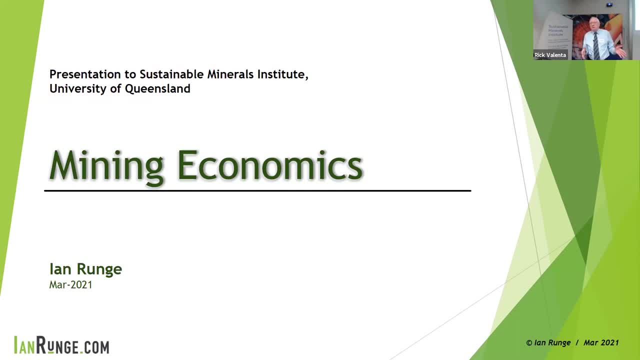 the second-hand value of it is nil. So it's the amount of capital at risk. in a mining case that's most likely much more. It's not just the total amount of capital, it's the percentage of capital- most of it- that's actually at risk. 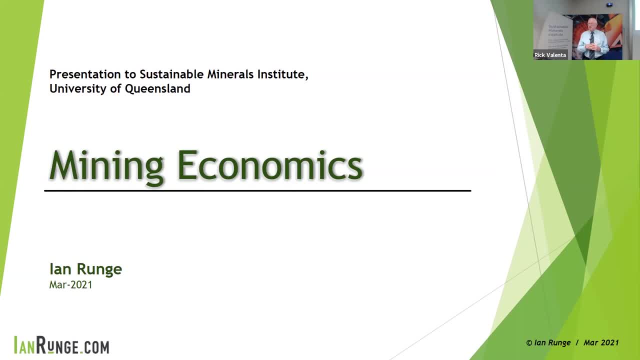 And in mining investments a lot more of our capital is at risk and therefore the sensitivity to actually giving them the go-ahead is much higher than a lot of other industries, you know, given the uncertainty about some new regulation. Thanks, My name is Claudia Moreno. 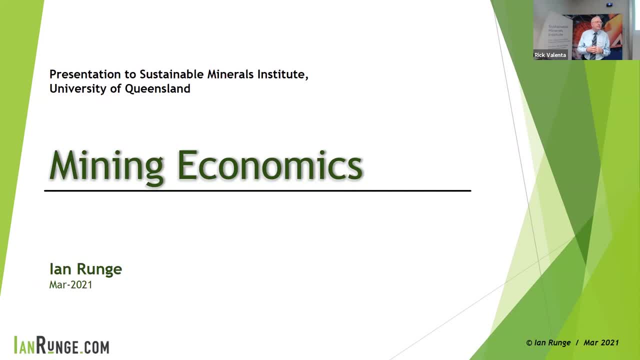 and I'm a PhD student at SMI and I would like to know if you have done any work including environmental costs in the planning of the mines besides their rehabilitation costs. I personally haven't done much of that because I haven't done much for a long time, but I think every 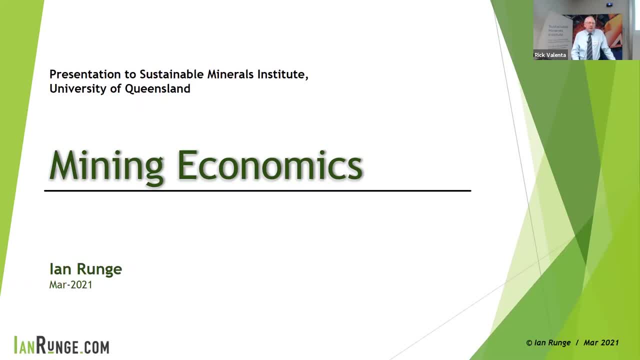 We do a mine plan, We'll have an environmental element to that plan and we would always be taking cognisance of that. actually, amazingly- Let me just not just say environmentally- Let's say you took my coal seam example. there There might be a thin seam of coal that's not economical to mine. 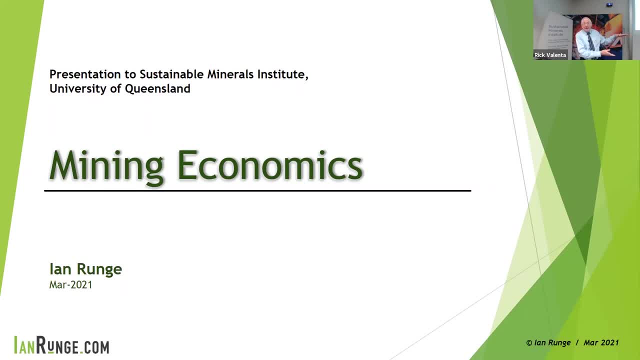 but I don't know of many or any companies that actually will. then They will try and mine that, because throwing it in the spoil is kind of wasting a valuable resource. And you see that repeatedly in mining companies, where they will make a deliberate choice.